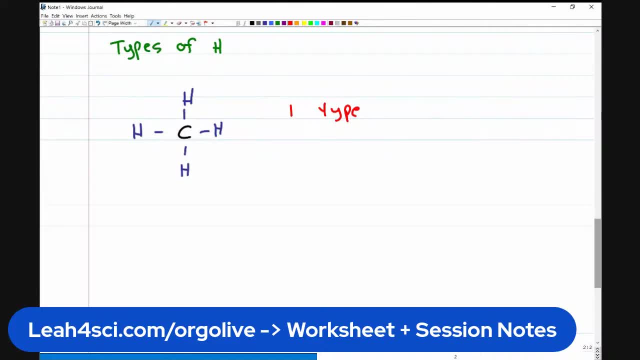 molecule and ask yourself, if I picked one hydrogen on a 3D model kit, so if I built this kit and all the hydrogens were the same color and I closed my eyes and picked one at random, if I closed my eyes and picked another one at random, would there be a difference? And if I picked another one at random? 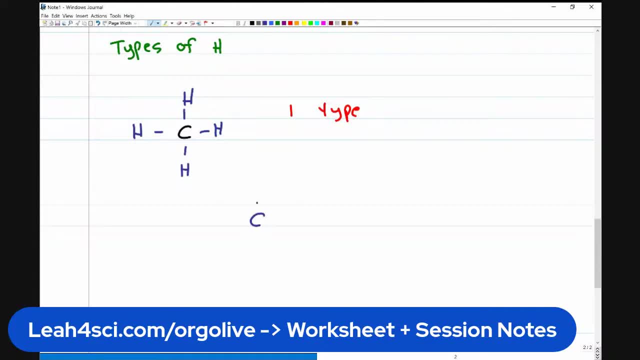 would there be a difference? And if I picked another one at random, would there be a difference? If you think about how the CH4 looks in three dimensions, it's a tetrahedron. How do I typically draw it? Like this: 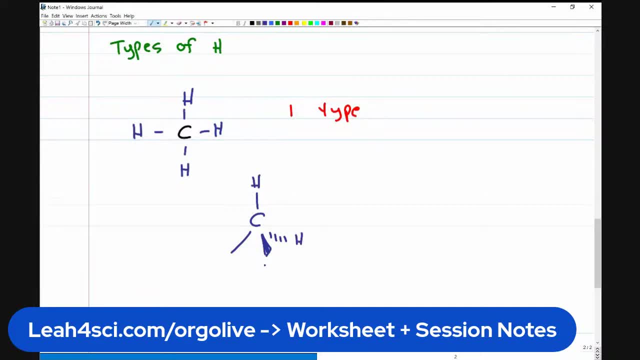 So we have a tetrahedron that is perfectly symmetrical. No matter how you spin this molecule, every hydrogen is exactly the same distance away from carbon, the same distance away from the other hydrogens, and that means they're all the same. 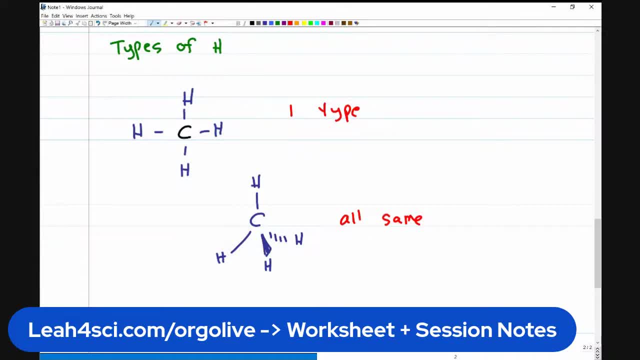 Because of the fact that we have a tetrahedron that is perfectly symmetrical, because I can spin this molecule around and not be able to tell one hydrogen from the next. when I throw this molecule into the machine that is going to read the HNMR, the machine that will 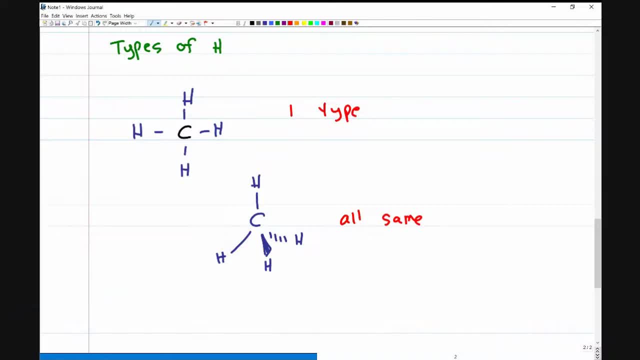 give me that graph, the machine also can't tell them apart. And as far as the machine is concerned- and I say machine because, again, I don't want to go into the physics behind it- I want to focus just on what you need to know for this topic. The HNMR machine apparatus cannot tell you the 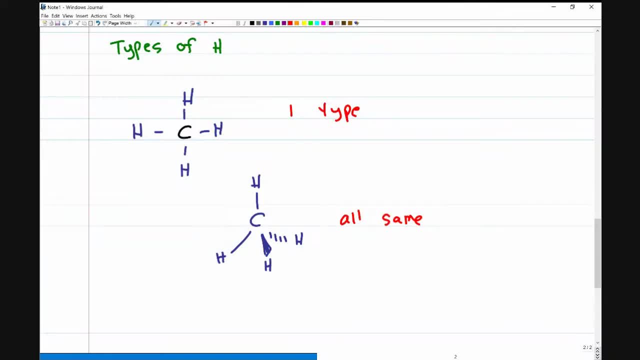 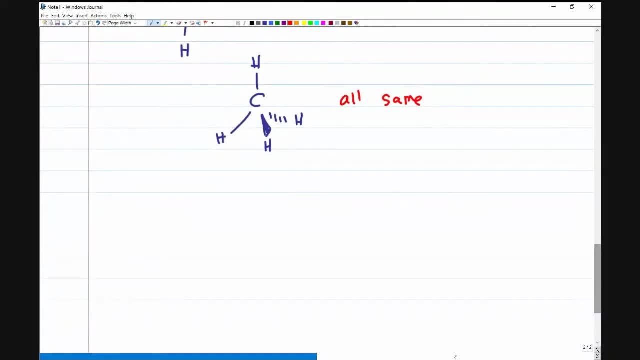 difference between the hydrogens and therefore we're not going to tell the difference between them either. That means we have just one hydrogen type. Okay, this was pretty simple, So let's crank it up a little bit. What if I have a molecule like ethane? Ethane, if you draw it out in. 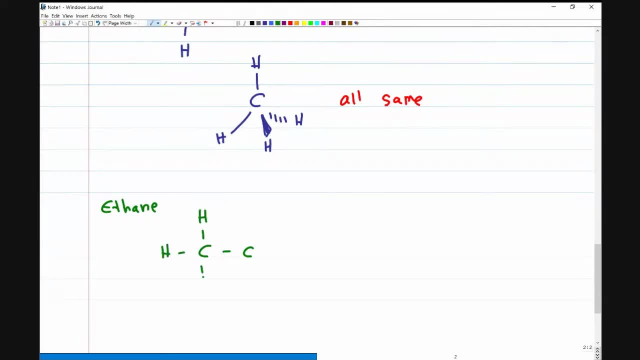 not in line structure, but just showing all the atoms, has a total of six hydrogens, three on each carbon atom. How many types of hydrogen on this molecule? Once again, we have just one type of hydrogen. Now this is a little different. It's not exactly. 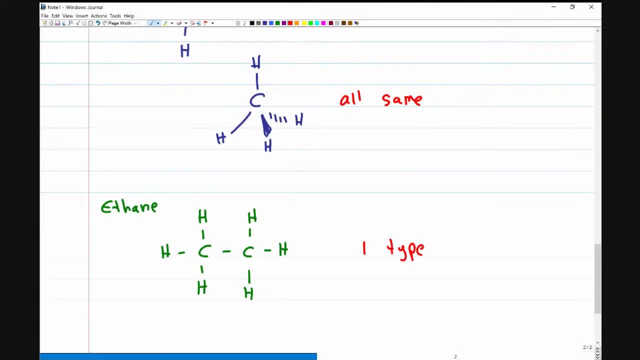 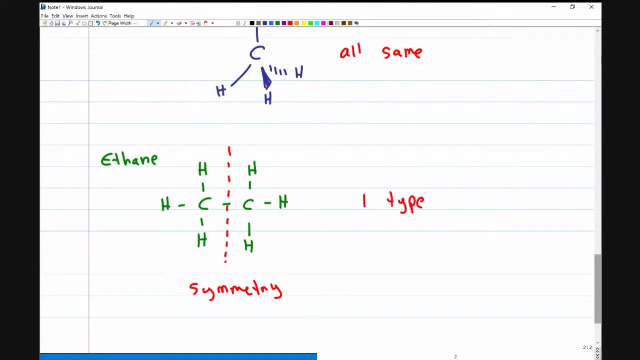 the same as before, where, coming out of the carbon, we had four equal hydrogens. But if you take this molecule and split it down the middle, you'll notice that we have symmetry. The symmetry means that, as far as anyone looking at a three-dimensional structure is concerned, the right and left half of 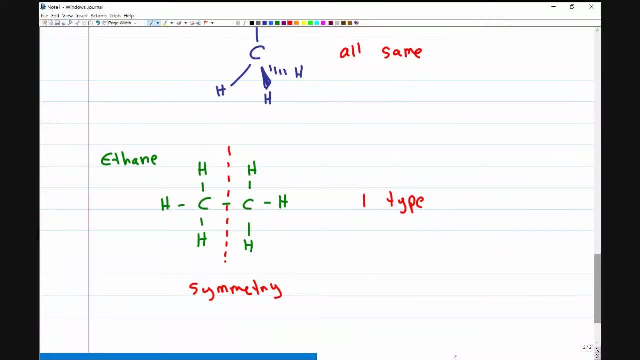 the molecule is the same. So if you take this molecule and split it down the middle, you'll notice that we have symmetry. The symmetry means that, as far as anyone looking at a three-dimensional structure is concerned, the right and left half of the molecule is exactly the same. And then if we 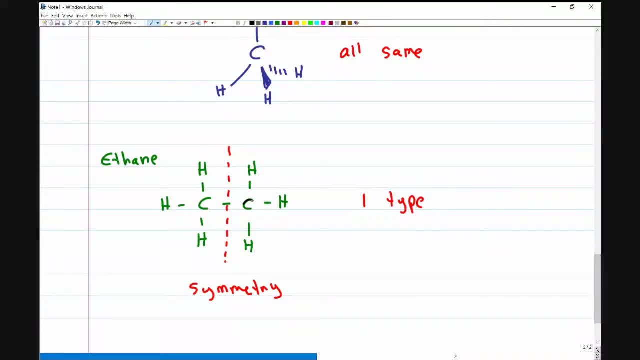 look at each of the equivalent halves, there's a carbon with a hydrogen coming out of it. But remember, this carbon is sp3. That means the hydrogens are all equidistant from each other. If I try to draw this in three dimensions, let's see if I can pull it off. So these will be carbon. 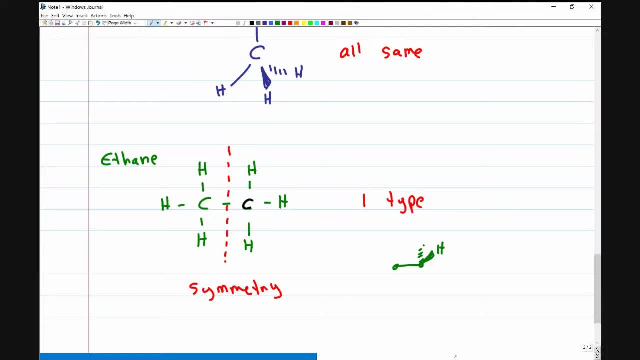 and I can put one hydrogen up out of the page one hydrogen up into the page one in the plane, like that, And let's do it this way, And I can spin these around because the hydrogens are exactly the same. You can't tell the difference between this one and this one And because of the symmetry in 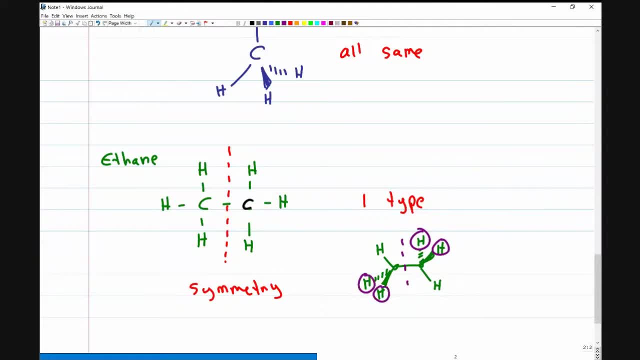 the molecule. you can't tell the difference between these two either, And that means, once again, we have just one hydrogen type and therefore one signal. If this is easy, so far, you're with me. so far, go ahead and give this video a thumbs up. 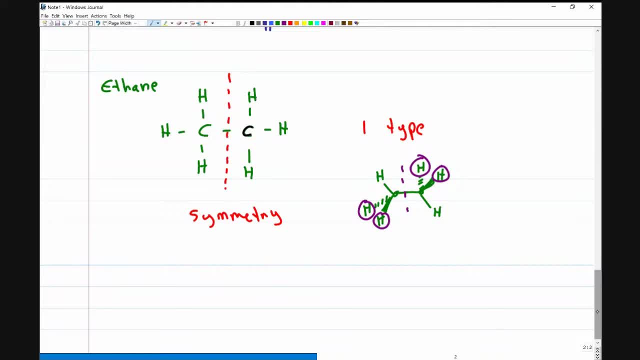 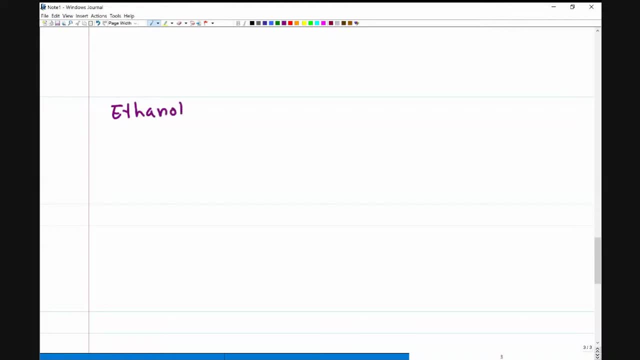 Let's see what happens if we change this molecule ever so slowly, where, instead of ethane, I give you ethanol. All I did was change it from CH3CH3 to give you CH3CH2OH. I just added an oxygen. If I draw that out now, how many types of hydrogens do I have? 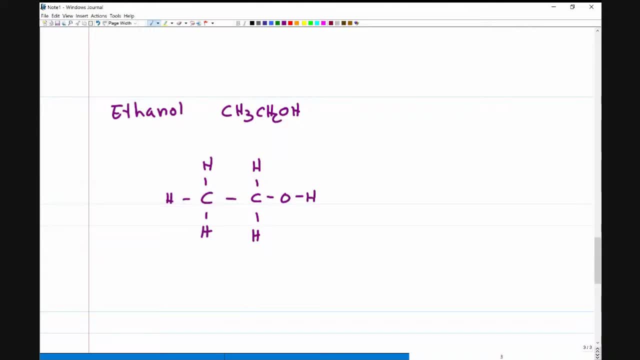 Now I have three. There's no longer symmetry in the molecule. And if there's no symmetry, I want to start looking at where the neighborhoods are Meaning. if a hydrogen is exactly the same as another, we call it the same one signal, But if there's something different going on, it's going. to have a unique signal. So if there's something different going on, it's going to have a unique signal, And if there's something different going on, it's going to have a unique signal. So if there's something different going on, it's going to have a unique signal. on the HNMR graph. 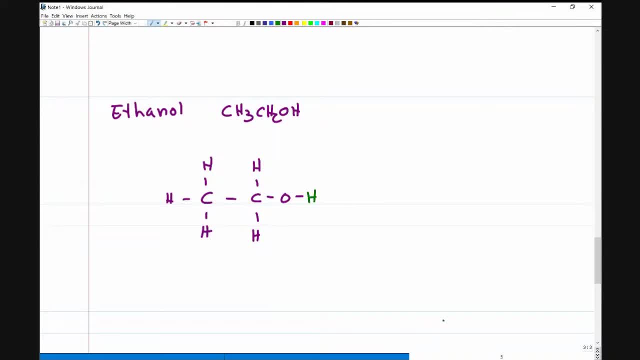 The obvious one is the alcohol, because the hydrogen sitting on oxygen is the only hydrogen sitting on oxygen. If we jump over one, these two hydrogens are exactly the same as each other because on this carbon atom, a hydrogen coming out of it is exactly the same as another hydrogen. 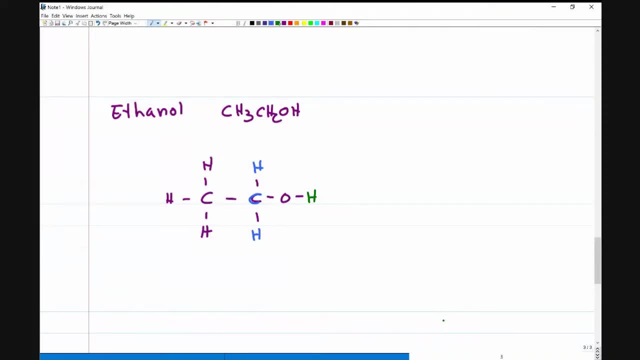 coming out of it similar to what we saw before. But if we move on over to the next carbon atom, we have a hydrogen sitting on oxygen, And if we jump over one, these two hydrogens are different. Because this carbon has three hydrogens, Let's mark them in different colors so we can. 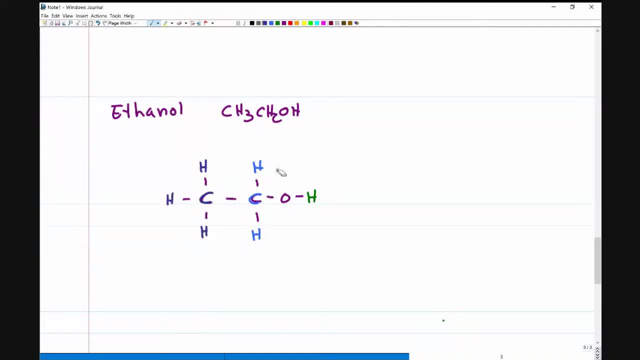 tell them apart. This one has three hydrogens. This one has two hydrogens, which is different from the hydrogen sitting on an oxygen. Three hydrogen types And this is going to be critical to differentiating this molecule on an HNMR graph. Are you with me? 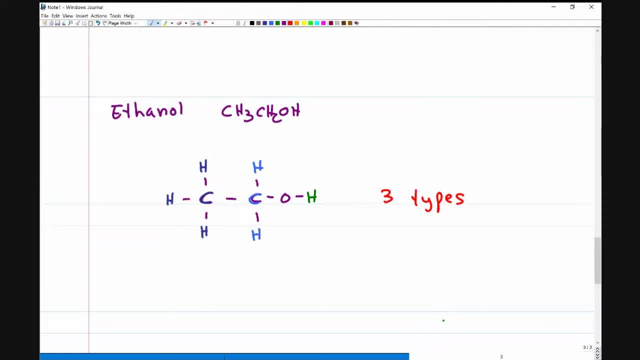 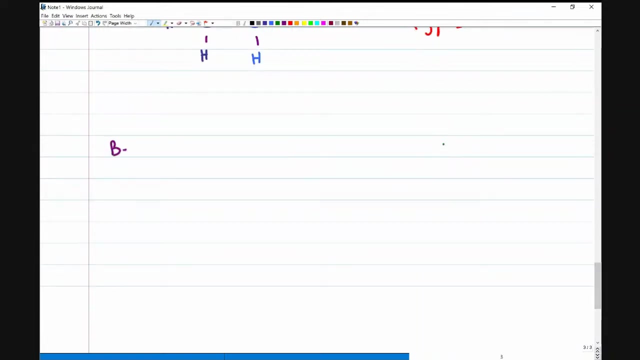 So far All right. If you are again, this should still be relatively easy. But let's bump it up and take a look at benzene. Benzene is an aromatic compound. Benzene is an aromatic compound with pi bonds on every single carbon for a conjugated system. 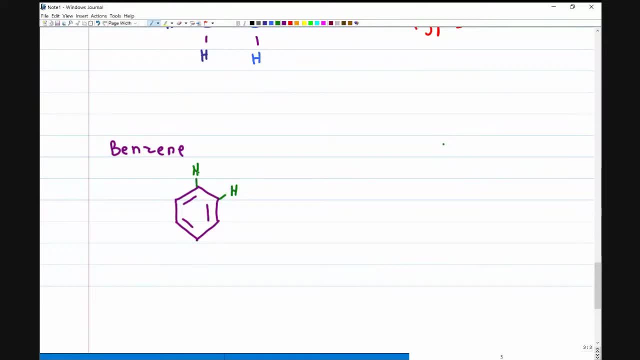 And benzene has a total of six hydrogens, C6H6.. If you built this in a 3D model kit, would you be able to tell the hydrogen atoms apart from each other? No, they're exactly the same. There's symmetry this way, this way, this way, However I slice it, there's symmetry in the. 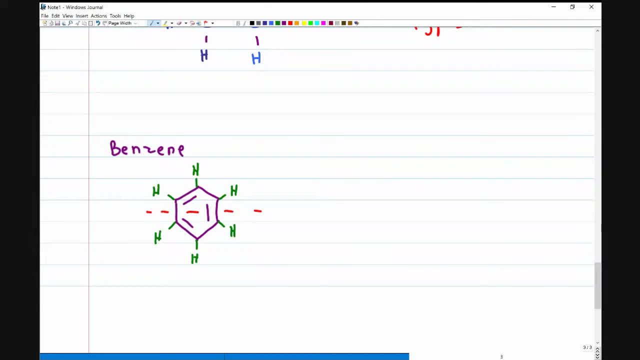 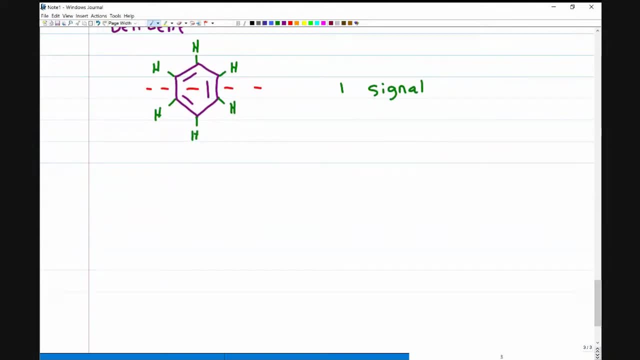 hydrogen is going to look the same And we have a total of one signal. What if I take this molecule of benzene, but this time I add a methyl group to it? How many signals on toluene, which is simply a sposethrol, add up to 15.. entre the two hydrogens: 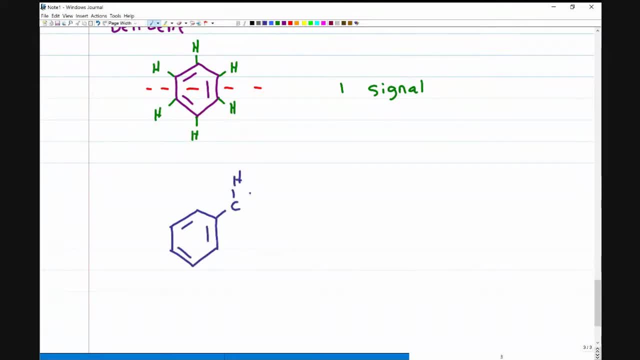 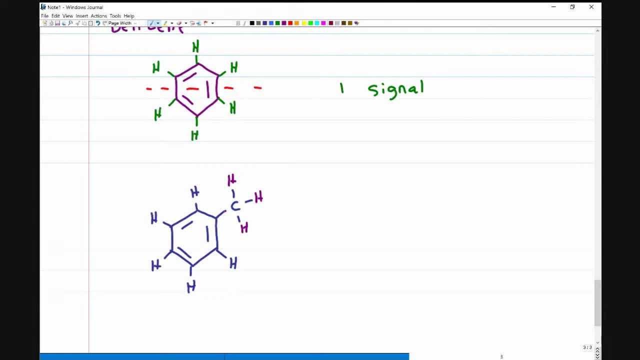 three hydrogens that look exactly the same. That right, there is an SP3 carbon. This bond can rotate. All the hydrogens look the same, But the symmetry here is not quite what it was before. The only symmetry I have now is this way, That means whatever I have on the top of the molecule. 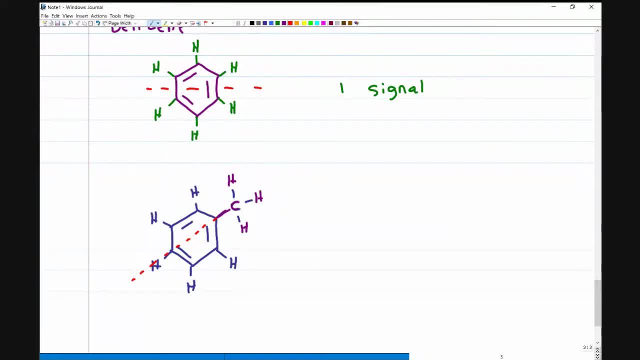 is going to be the same as the bottom, but the right and left are no longer the same, So let's break it down. The first set of hydrogens that are equivalent are the hydrogens directly near the methyl group, because these hydrogens live in a neighborhood that is one away. 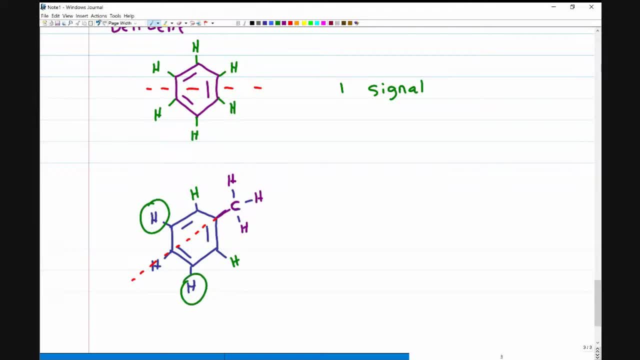 from a methyl and one away from a hydrogen atom. If we jump on over to that hydrogen atom, what is the neighborhood that these live in? Notice they live in the exact same neighborhood because of the symmetry going down the middle: The neighborhood of the light blue hydrogen. 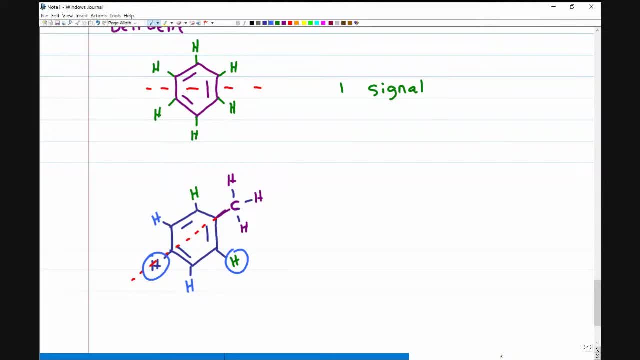 is a hydrogen and a hydrogen. It has a hydrogen on either side, So the hydrogen is going to be on either side. And then this one right here: well, it also has a hydrogen on either side, So it's a very similar neighborhood. This is where it gets a little tricky. Some professors will. 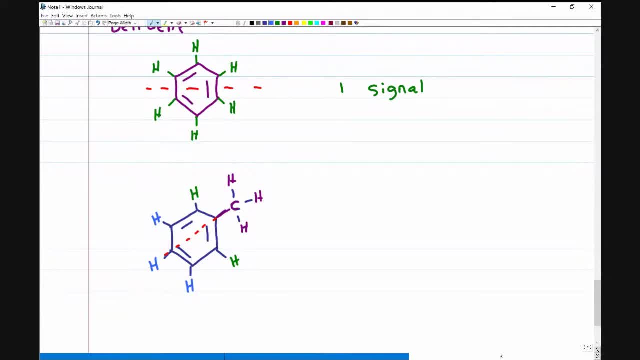 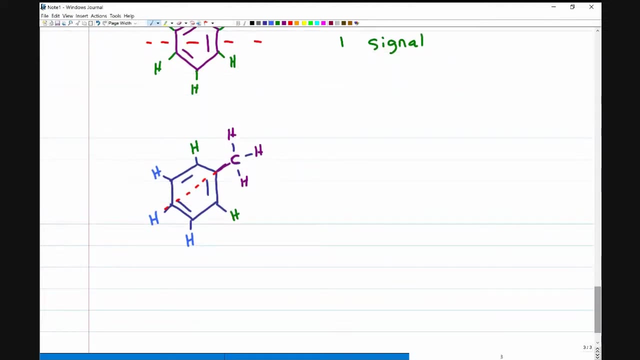 count it as the same. Some professors will count it as different. I have seen both as the correct answer And on a graph. it will be very hard to distinguish between them. So just a heads up there. Let's do one more. So this one, we'll call it three types. 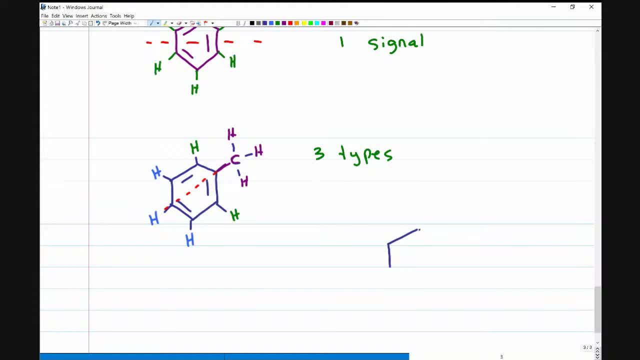 And why not one more benzene, just to make sure we're comfortable with it? What if this one has a carboxylic acid here and we'll put an alcohol here? How many hydrogen types do you see? Well, let's see. First, I like to look at my functional groups. If I have a carboxylic acid, 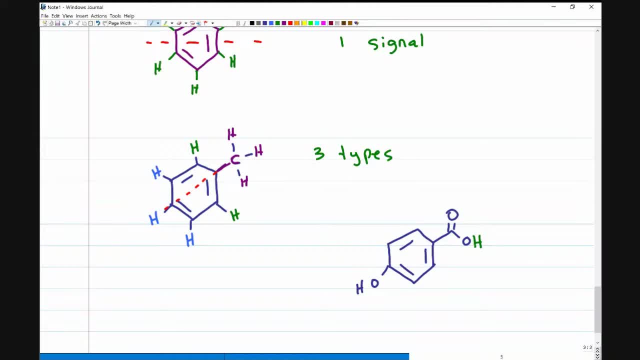 that's a unique hydrogen right there. If I have an alcohol that is a unique hydrogen right there, There's no other like it. The benzene ring itself has a total of one, two, three, four hydrogens. But there's no symmetry here because one side of the molecule has a carboxylic acid. 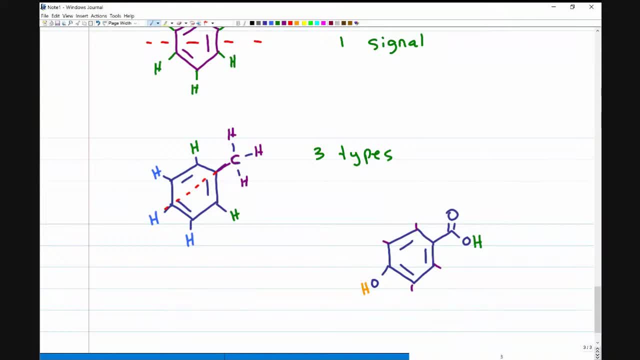 the other side has an alcohol. However, there is symmetry going this way, And that means the top and bottom half are the same for a total of well, let's see, These two hydrogens are the same. And these two hydrogens are the same. What makes them different from each other? 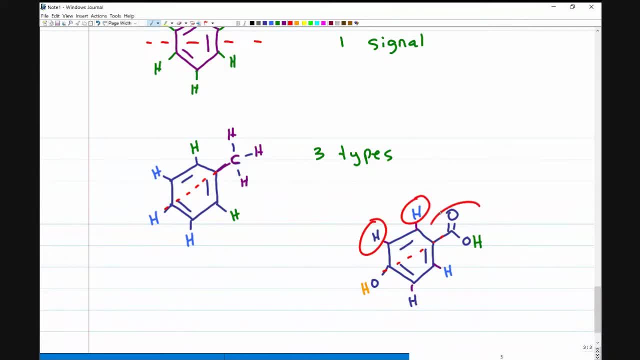 This hydrogen is in the neighborhood of a hydrogen and a carboxylic acid, as is the one on the bottom. This hydrogen is in the neighborhood of a carboxylic acid and this hydrogen is in the neighborhood of a carboxylic acid. 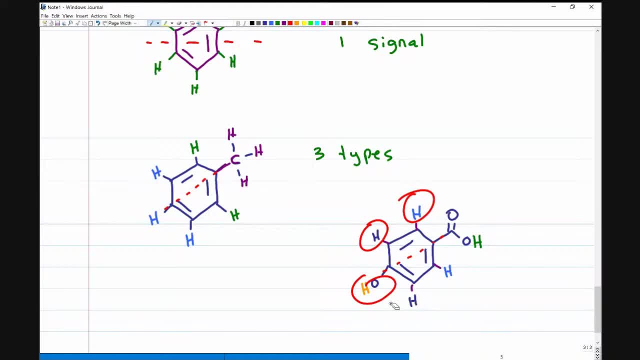 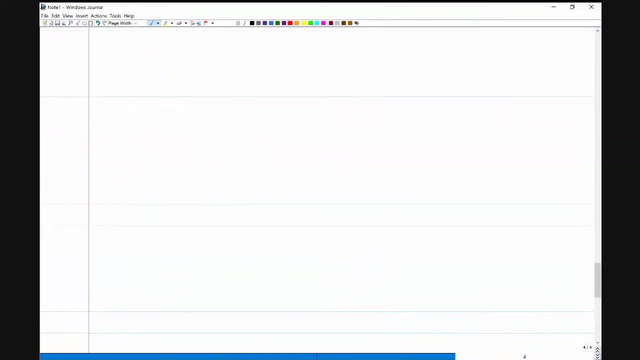 of an alcohol and a hydrogen. all right, any questions on this, let me know in the comments. otherwise are we all set on hydrogen types and the concept of hydrogen neighbors? are you ready to see what it looks like on a graph? now the practice questions we're working on. I will have even more questions for you on this and everything. 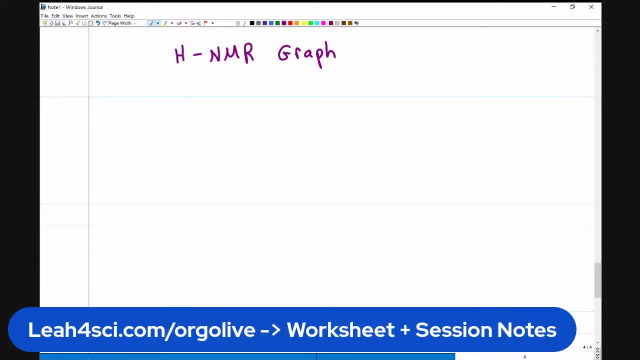 we discussed today. if you want to practice, you just have to sign up right here and after we're done, you'll get the worksheet and the session notes. if you sign up after the recording is already posted on YouTube, same thing: you sign up, you'll get the worksheet and the session notes. so let's 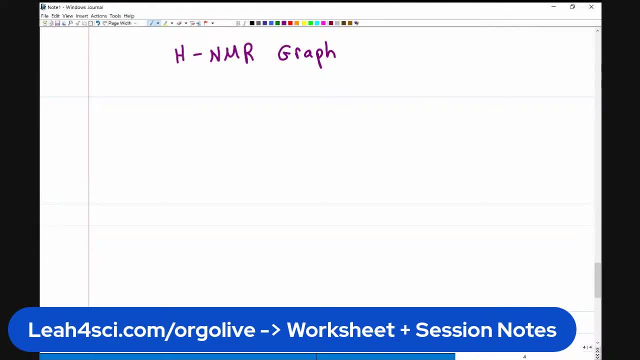 take a look at the graph. the hydrogen's don't simply just show up on a graph. it'll typically look something like this, with a lot of random bumps and things and chicken scratch. the key is to figure out what these things actually are and what they are, and what they are actually are and what they are actually. 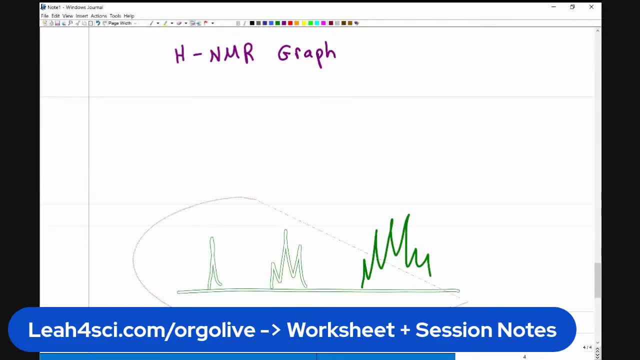 mean and specifically what we're looking at here are the splitting patterns. so we talked about the hydrogen types that will give us the splitting, which I'll show you in a moment. but the single bump, the triple bump, this crazy multiple set of bumps, this right here is very important to understanding what 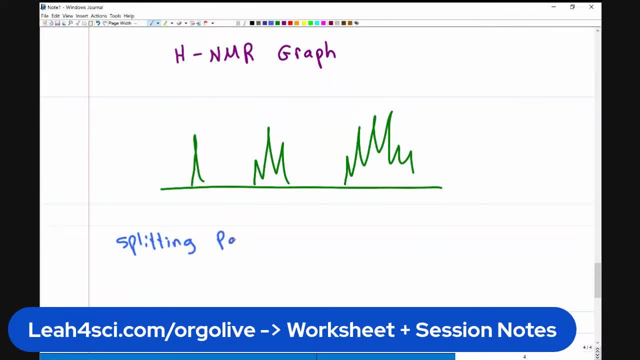 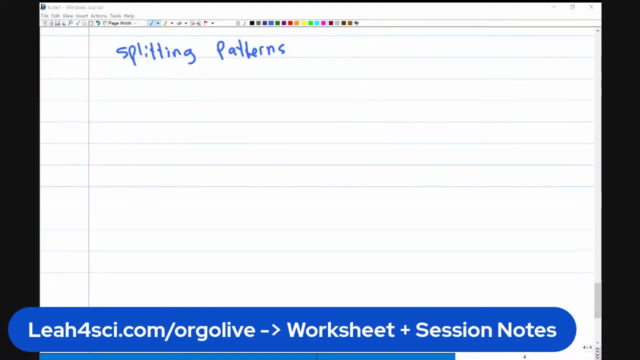 we're looking at in terms of not just the hydrogen, but what is next to it. so let's take a look at splitting patterns for these different groups. the first one is just a single peak going up and coming back down because it has a single head. this is called a singlet, based on the way this 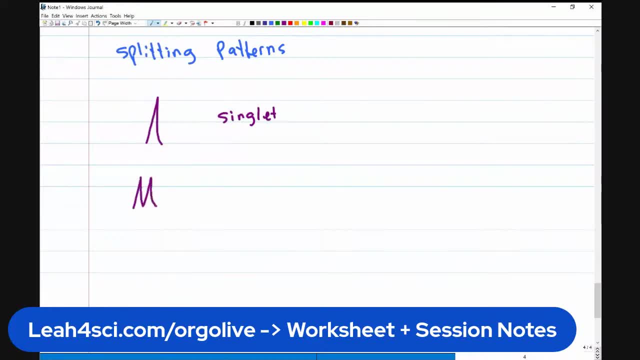 one is named. what would you call one that has a double head? two peaks you. this is called a double. what happens if I draw a triple? if we're going with the pattern of what it is with an le T, then this should be called a triplets. if I Mérito. 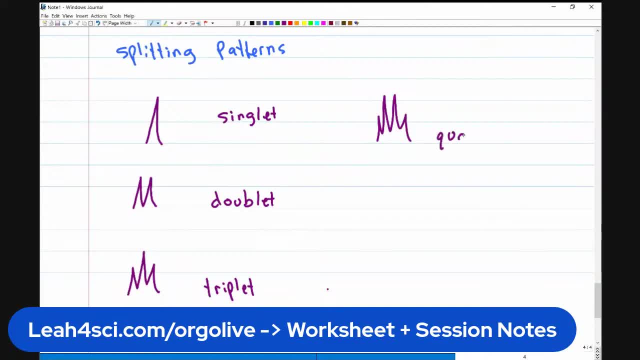 i2 draw four, called a quartet. If I draw five, this is called a quintet. And honestly, after four they tend to get lazy. So if you see something like this on the graph, they don't even count the peaks, They're. 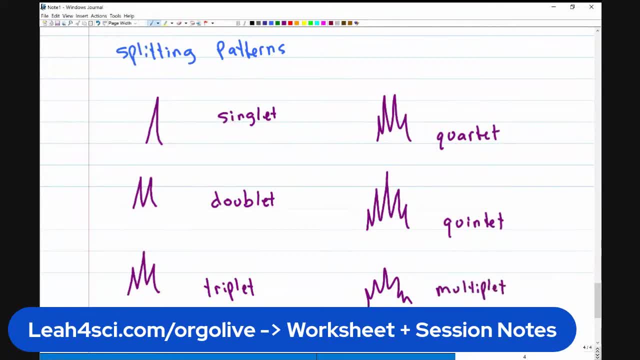 just going to call it a multiplet And, depending on the graph that you're looking at, the multiplet will be greater than or equal to five peaks, So six, seven or more. they'll typically just call it a multiplet because it's got multiple and sometimes hard to differentiate. 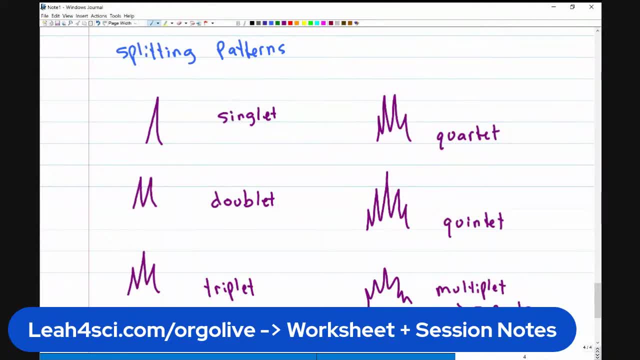 All right. so what does this actually mean? Again, I want to focus just on the tactical- what you're actually going to apply- rather than the detailed science behind it. The way I want you to think about this is if you're going to draw a quartet. 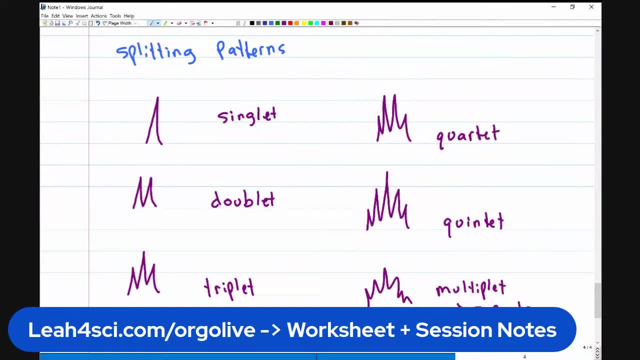 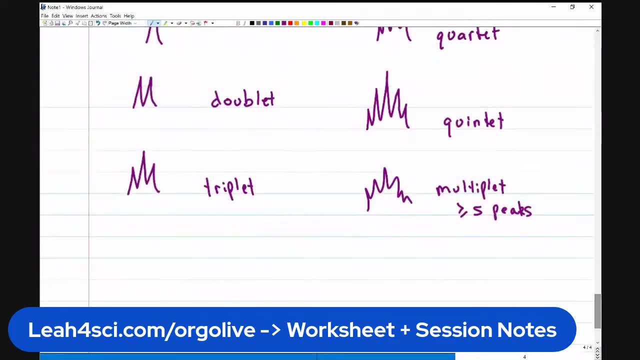 every peak represents a hydrogen potentially being pulled in different directions by its neighbors. We're going to call neighbors just the letter N, And so anytime I write the N, you know I'm talking about the neighbors. And what the neighbors are trying to do is simply. 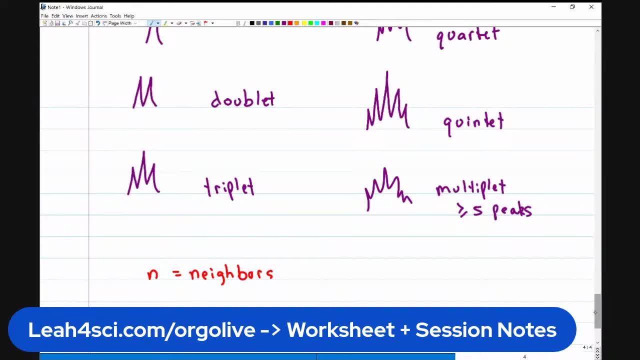 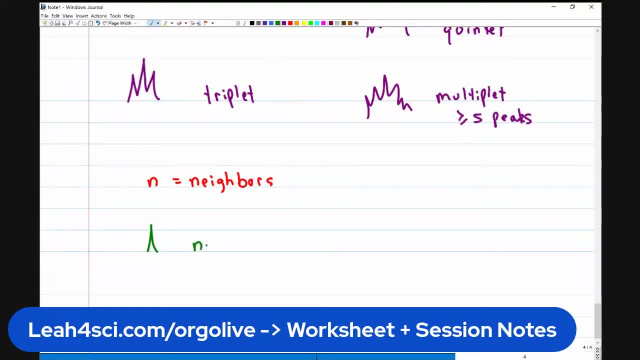 pull the peak in different directions. And so if I have a hydrogen sitting on a molecule minding its own business with no neighbors, N equals zero. And then I bring in a hydrogen, The hydrogen is going to try to pull this peak apart in two different directions. So this right here has N equals one, We bring in one. 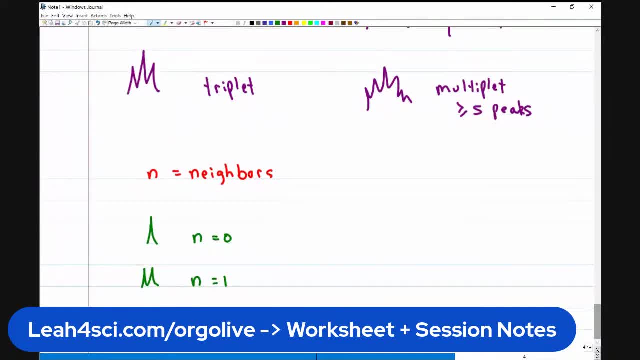 neighbor, it pulls it in two directions. Based on this pattern, how many neighbors do you think this one has? if you see a total of three peaks on the graph, It should have two neighbors. A quartet will have a total of three neighbors. A quintet will have a. 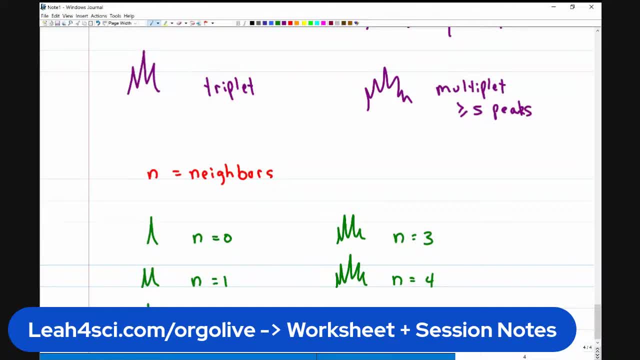 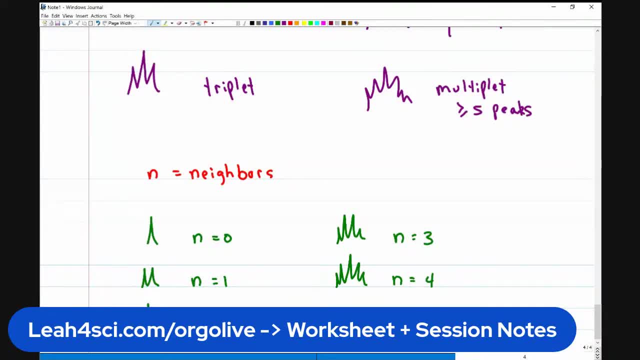 understand. So all this goes into boring detail. I'm looking for the tactical. What do I make of the thing I see on the graph? And this is all I'm looking at. Based on the pattern that we see here, we can come up with a very simple equation to follow. 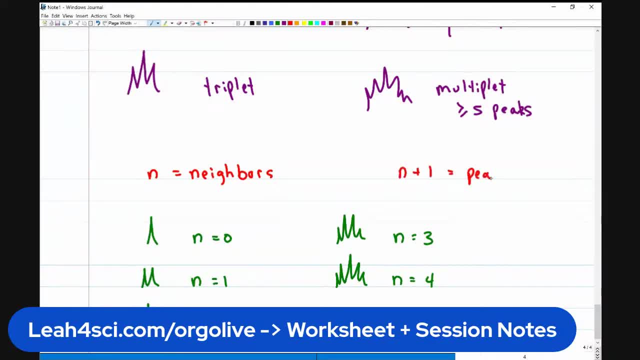 And that is N plus one is going to be your peaks, Your neighbor plus one. So this one has zero neighbors. zero plus one is one point four peak. this one has one neighbor, n plus one. one plus one is two peaks, and so on. 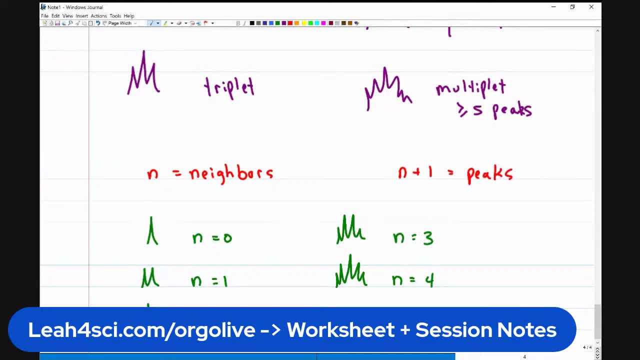 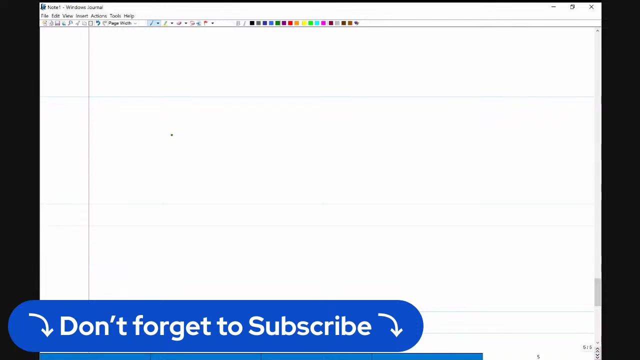 and so on and so on. any questions on this? if yes, go ahead and type it in. all right, so what happens if you're looking at a molecule on a graph and you see something like this? quick reminder: n equals how many neighbors? again, we're using the equation of n plus one is going to give me the number of peaks. 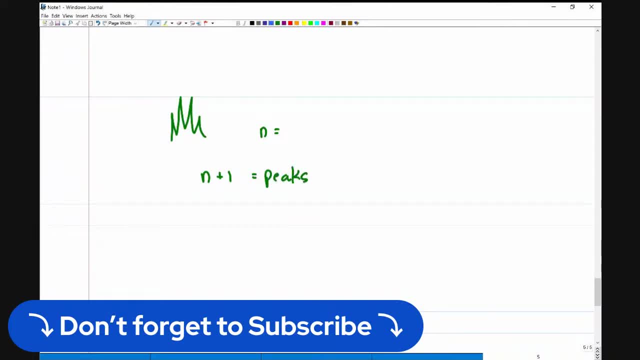 if we're using n plus one equals peaks, then what happens is, if you're looking at a molecule on a graph and you see something like this: When you see the number of peaks, you just do: peaks minus one is equal to neighbors, And so the peaks here. I just count the tips. 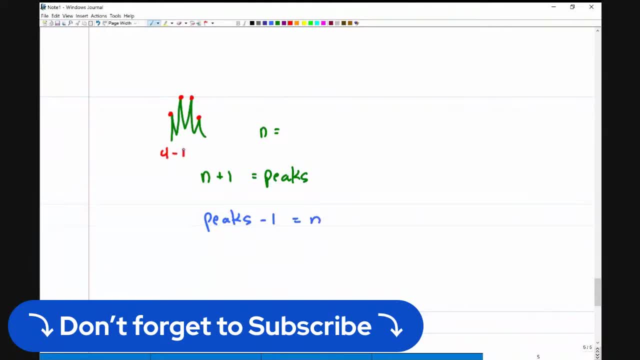 One, two, three, four, Four minus one equals three and equals three. I have three neighbors. What does three neighbors actually mean? We keep talking about neighbors and splitting, but what is a neighbor? Remember, since we're looking at HNMR, we're looking at hydrogen neighbors. 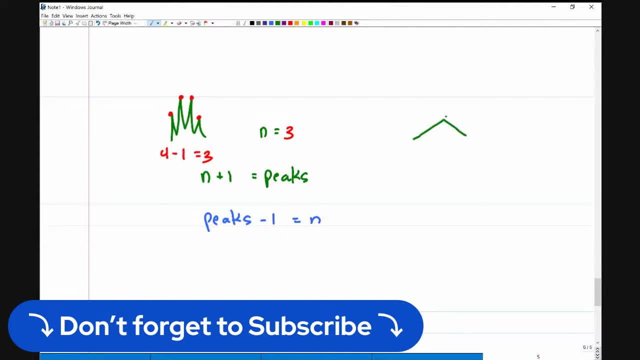 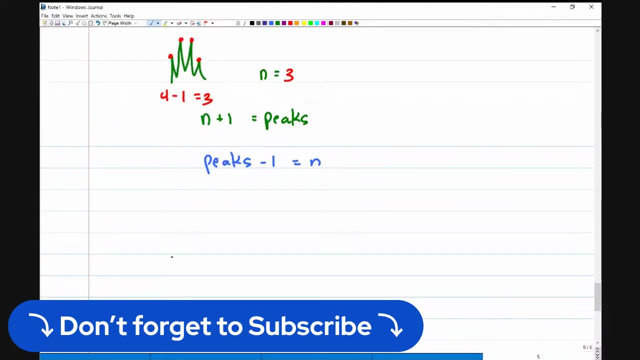 So if I have a molecule that looks like this and I have the green hydrogen, that's equivalent. so they are technically one peak. And you know, let's keep it simple. for this example, Let's draw one here. If I have this molecule right here with an OH layer, 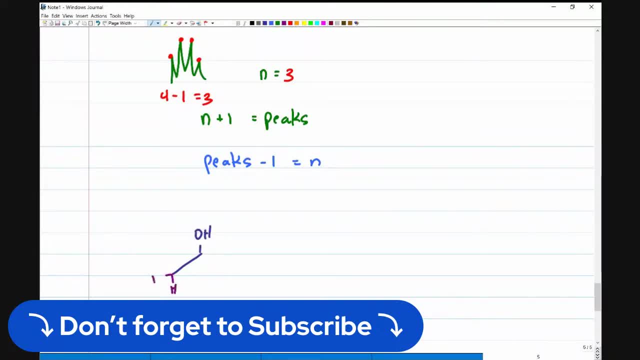 like that. this is the CH3 that we saw before. The purple hydrogen is technically one type of hydrogen, So it would be one peak if it was all by itself. But the neighbor, the carbon directly attached to the carbon holding it, the purple carbon, is the one that's holding the hydrogens in question. 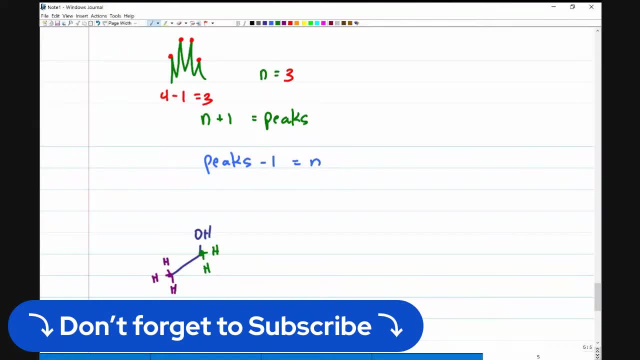 Directly attached is the green carbon, And the green carbon has two hydrogens. That means we have a peak. That is my one. N plus one is going to give me my peak. Now, in this case, N is two neighbors. 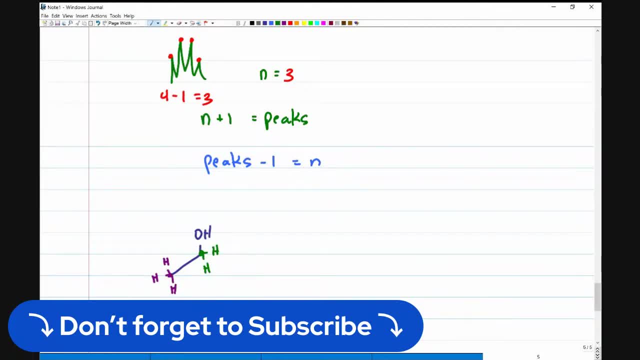 Because the purple set of hydrogens have two neighbors, the peak is going to be a triplet. I'm going to have a total of three. We talked about CH4 earlier. What kind of peak would you expect to see on a graph For CH4.. 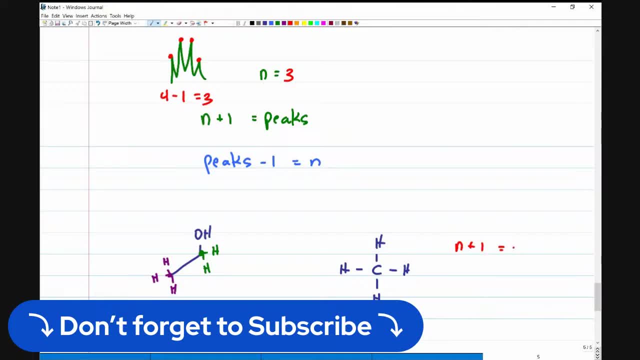 Remember, N plus one equals peaks. We have the blue carbon. Well, that's not blue. We have the blue carbon that is holding all the hydrogens. The hydrogens are equivalent. That would give me one peak. We have no neighbors. 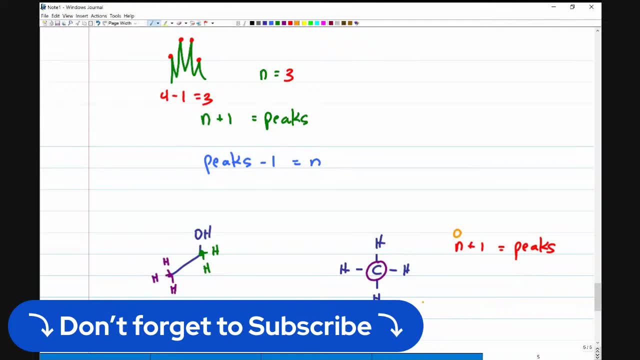 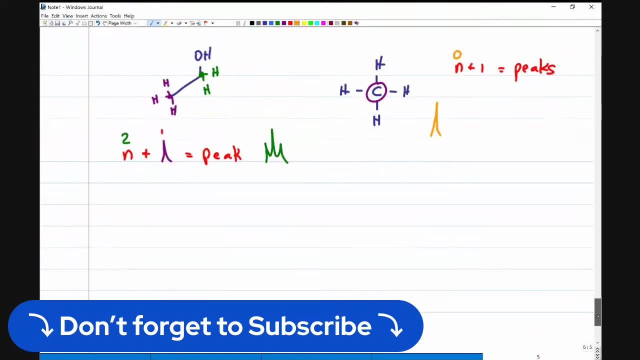 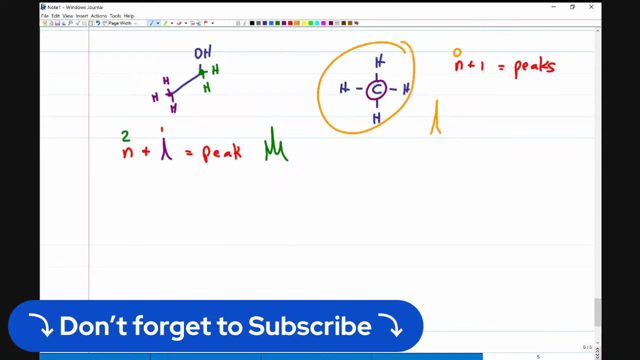 Zero neighbors And zero plus one is going to give me one single singlet. peak for this molecule Is the only way for me to have a singlet. this right here Meaning: does the molecule have to be methane for it to qualify for having a singlet? 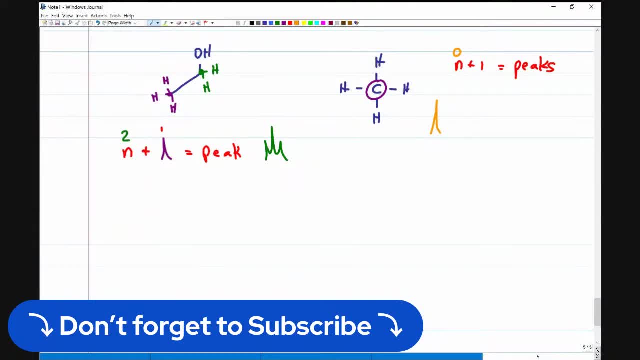 Or can I have a singlet in a different, larger molecule? All right, And I do see some questions coming in. Where did that go, Okay, Okay. So let's look at the blue hydrogen molecule and see if it applies to cyclic compounds. 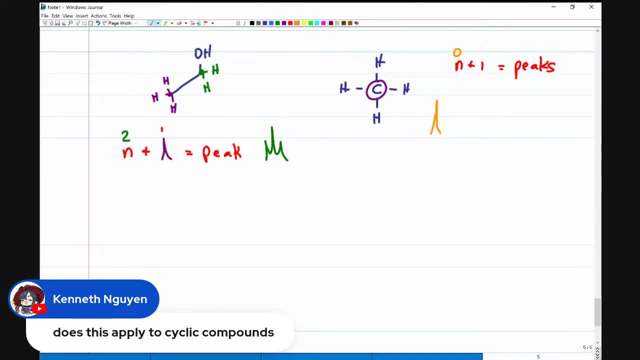 Absolutely linear or cyclic. If we have a carbon with hydrogen and then neighboring hydrogens, the same thing applies. So let's first answer this one and then look at a cyclic example. Well, we already said, this is a singlet, but it does not only have to be methane. 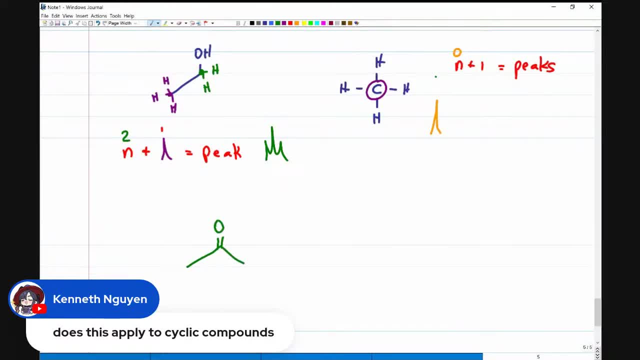 Because, for example, I can have a molecule that looks like this: Notice there's symmetry down the middle. That means each of these blue hydrogens have a molecule that looks like this: Notice there's symmetry down the middle. It just looks like this: 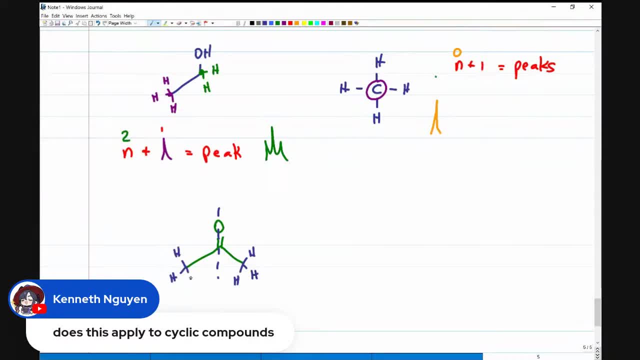 Notice there's symmetry down the middle. Notice there's symmetry down the middle. What's the key? leave of non- WOW ingredients. I know we can combine, but there's a misunderstanding. I saw someone say they took the capital N and now it's Ikf-1, QuA-1. зачем they look the other way? 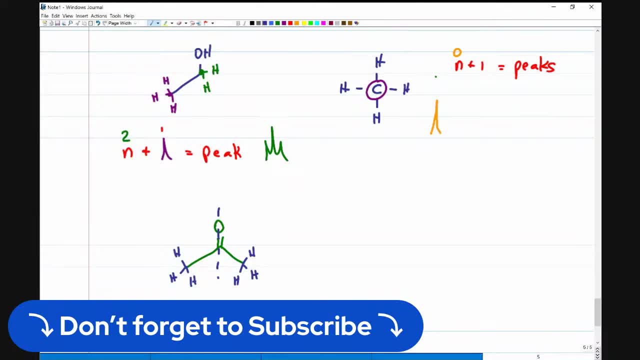 If these are exactly the same, I have six blue hydrogens that are equivalent and N equals zero. They have no neighbors, and that means I will have one singlet representing a total of six hydrogens and nothing else on the graph. Okay, so let me go back to this question on cyclic compounds. 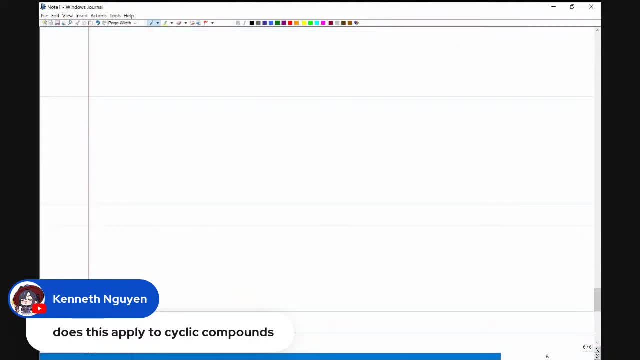 Let's say I have a molecule that looks like this and we'll have a CH3 right here If I'm looking at this blue hydrogen. how many neighbors does this blue hydrogen have? So N plus 1 is going to give me my peaks. 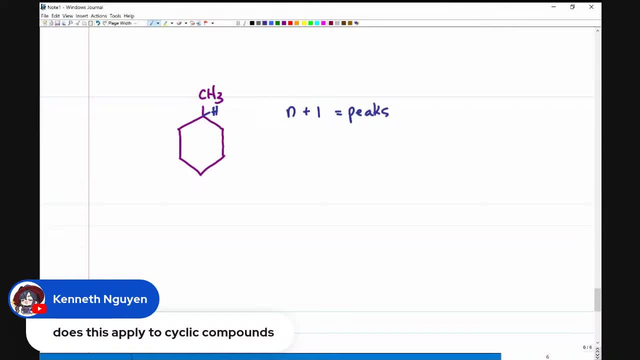 and this 1 is the signal for the blue hydrogen, because you always start with one peak. Let's count our neighbors. I have a total of 3.. 2 and 2.. Now I should draw these in different colors because they're all unique from each other. 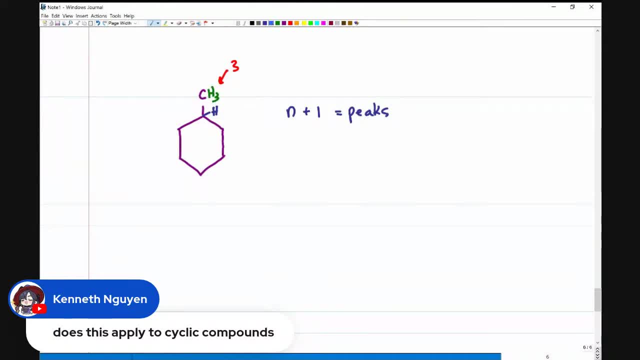 So the methyl group has three unique hydrogens and because of symmetry in the molecule, these are the same and these are the same right there. So that means I have a total of 2,, 4,, 7.. Neighbors are 7.. 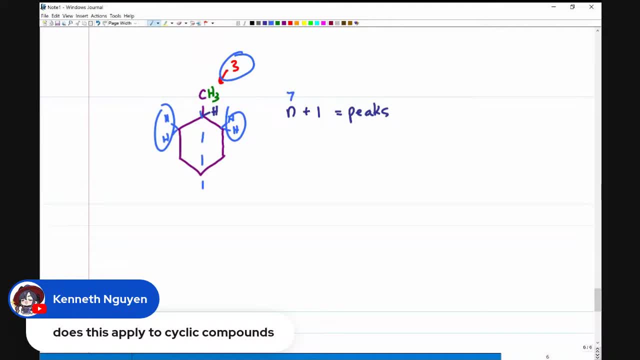 7 plus 1 is peak. I'm going to have an 8 peak and this is where you just say M, M, M for multiplet and it would be a total of 8.. So 1, 2,, 3,, 4,, 5,, 6,, 7,, 8.. 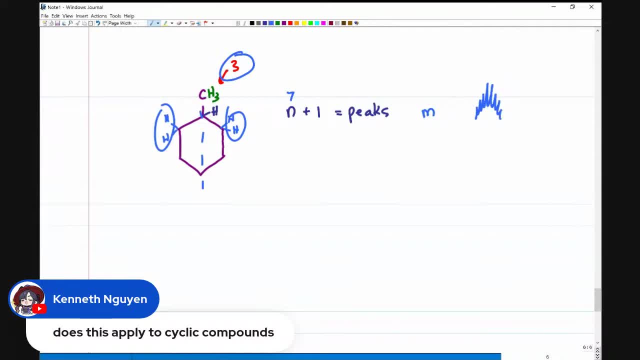 Typically you won't be able to make out how many tips there are, but we'll assume it's correct when it's really, really tiny. It'll look like this on your actual graph, where you can't make out what's going on. 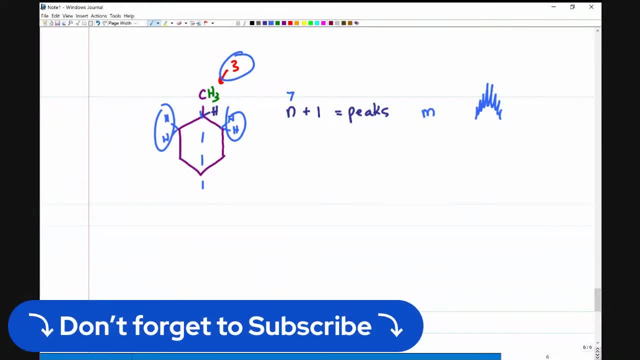 Then you just call it a multiplet. All right, If you have any other questions on this, go ahead and type it in. What happens? How many neighbors then for a molecule that appears like this on your graph? This right here is a trick question. 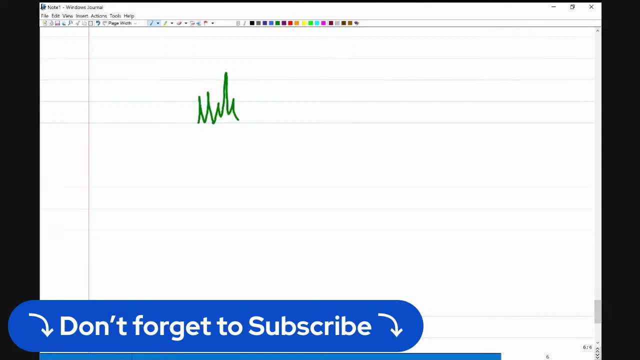 The reason this is a trick question is because when you're looking at a graph, sometimes the peaks are all on top of each other, and in this case, this is not one peak, This is actually two peaks, and the two peaks are as follows: 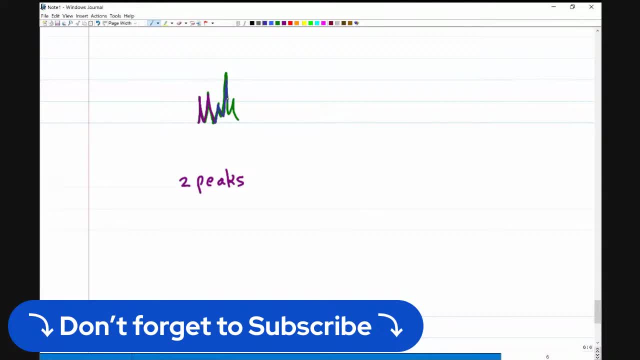 I have a doublet right here and a triplet right here. You're going to see these- maybe not very, very often, but often enough- And the way I tell the difference between this right here, which is two different peaks for a total of five, somehow. 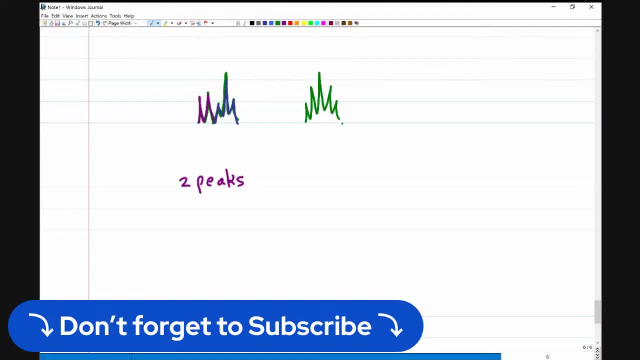 and a molecule that actually, that actually has five peaks, is what I call the hat trick. Now, the science behind this, the math behind this that we intentionally skipped, is showing you how to get the splitting patterns. but it's the way that the molecule splits, is always going to form some kind of almost like a pyramid. 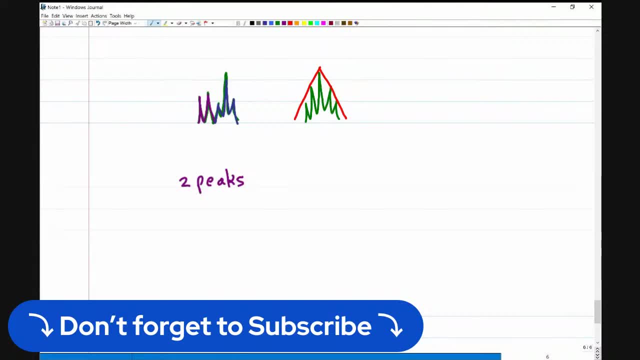 where the tallest ones are in the middle, and then they're shorter and shorter, going out to the sides, And so I call this a hat trick, because we're just putting a hat on the molecule. It has to go perfectly, So let's go back to the page where we drew them all out. 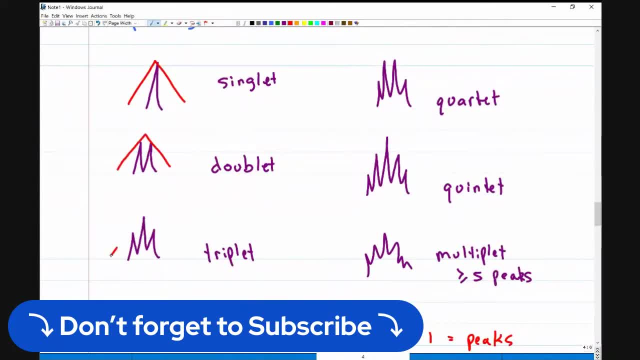 Watch, I can put a perfect hat on each one, And when you have a messy graph, this is very, very helpful to be able to do, because you can tell that the tallest peak, the tallest part of the peak, is in the middle. 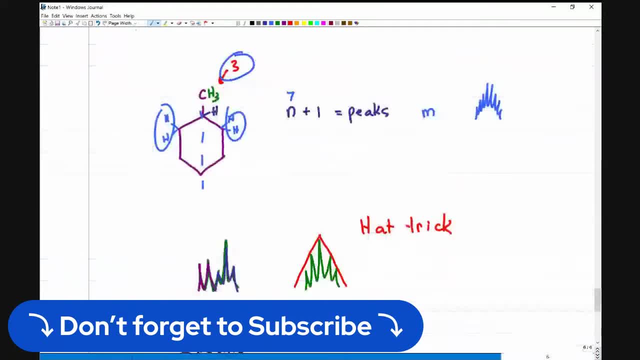 and then it gets shorter and shorter as it goes out, which is very different from what I have here, which is really This peak right here and this one right here separated. Is that clear? Does that make sense? Question: What you are saying is that symmetry plays a huge role. 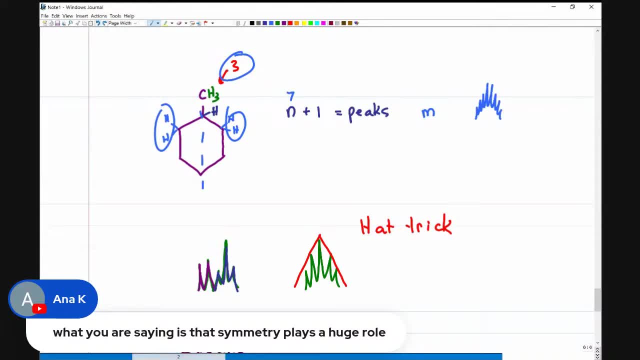 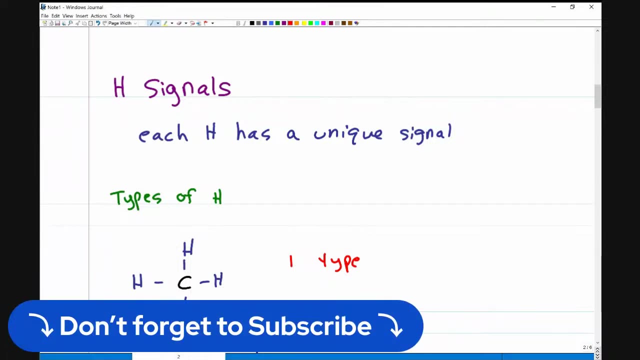 Yes, because symmetry makes the hydrogen atoms exactly the same. Notice, there's symmetry here. Therefore, you cannot differentiate the hydrogens, And on the graph you won't be able to differentiate the hydrogens either, because they look exactly the same. Great question. 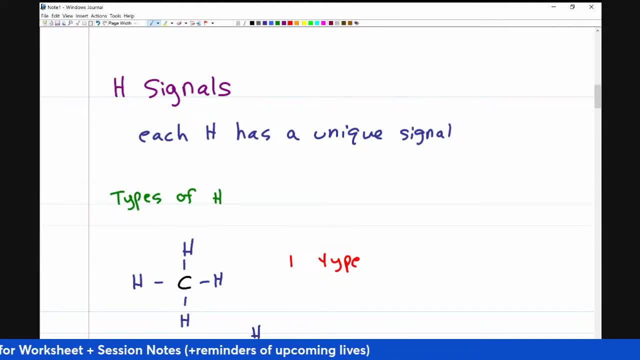 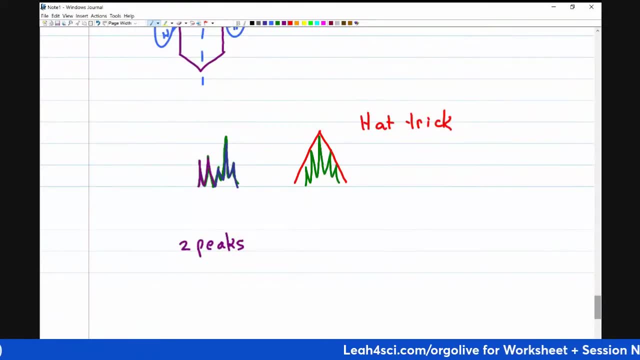 I'll put even more practice for this on the worksheet. So if you want to do more practice for signals and for recognizing how many peaks and neighbors, make sure you sign up here And let's continue. Are you ready to see this on a graph? right? 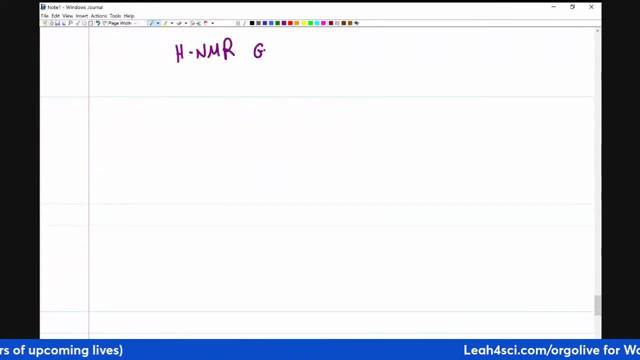 Isn't that what you came for? Let me know in the comments. You just came to see the graphs because that is all your professor cares about. Everything else was just leading up to this point. Let's see a graph already, But first we have a question. 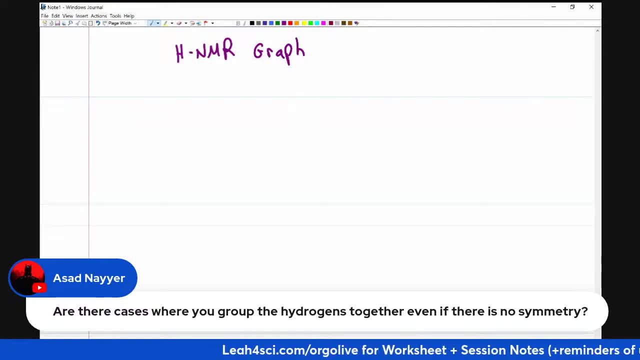 Are there cases where you group the hydrogens together even if there is no symmetry? The only time I've seen that happen is when you have a big molecule and you happen to have a graph where the peak shows up here and the peak shows up here. 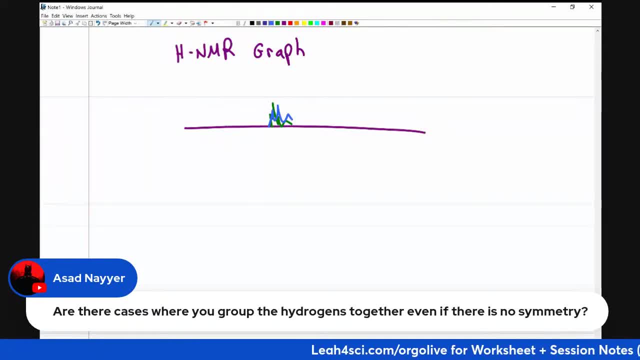 So they're not necessarily grouped. They just happen to sit on top of each other and get in each other's way. Those tend to be the trickier examples, though, So hopefully that answered your question. All right. So what are we looking at with an HNMR graph? 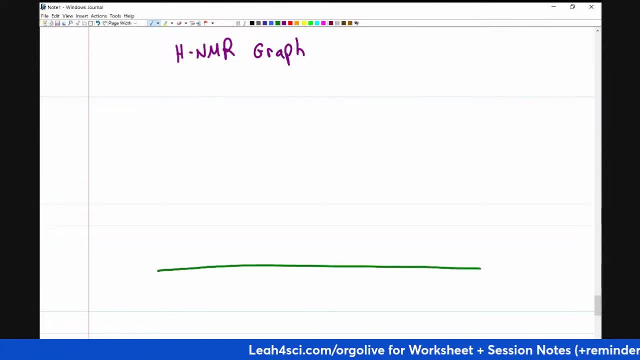 As with any graph, we need our axes. Now this one. you're not going to see X and Y, You're just going to see it written out like this: Sometimes you're only going to see a part of the graph, but obviously the part that matters. 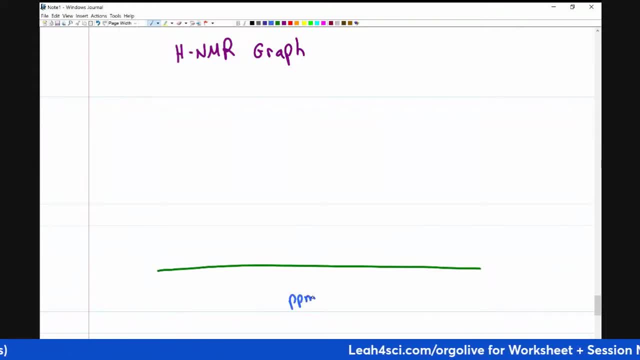 The label down here doesn't really matter, but it's ppm- parts per million. This is a sample where you have lots and lots of samples dissolved in a solution, And then you're going to see the numbers on the right from zero and on the left going all the way to 12, with everything in between. 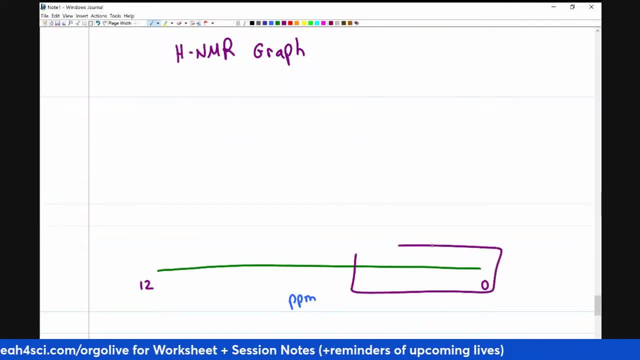 But sometimes, if the molecule is simple, the graph may only go till five, and that's fine. So zero, one, two, nine. I'm just going to put dot, dot, dot to 12, because I clearly didn't space that enough. 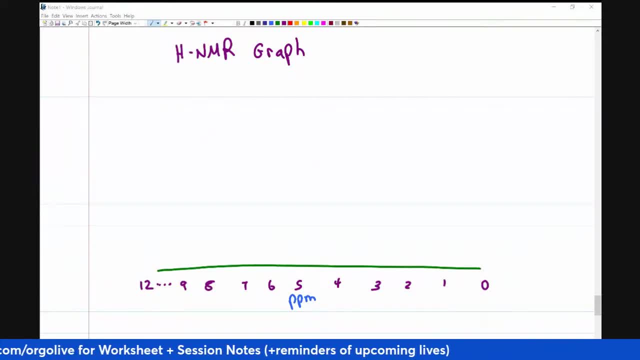 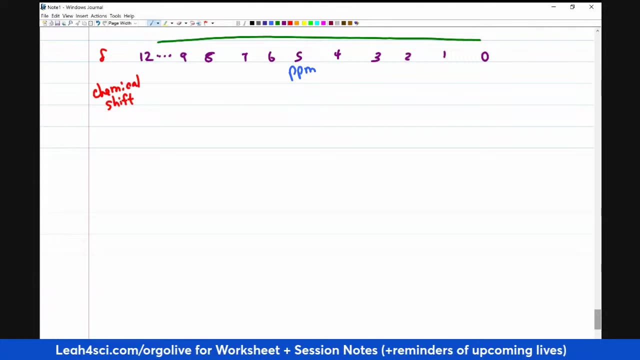 And the number that we're looking at. this is the delta value, And the delta value tells us the chemical shift. Let me know in the comments if you have taken the time to memorize chemical shift values such as something like this. I just grabbed this off the internet. 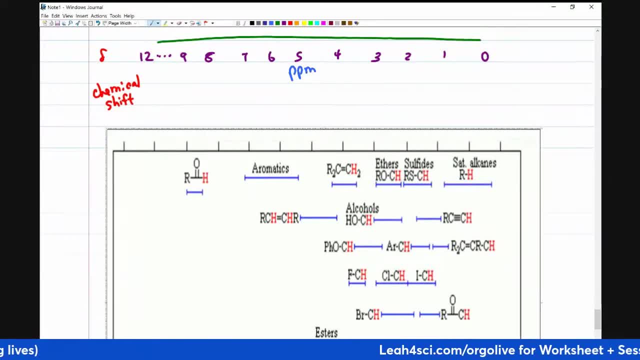 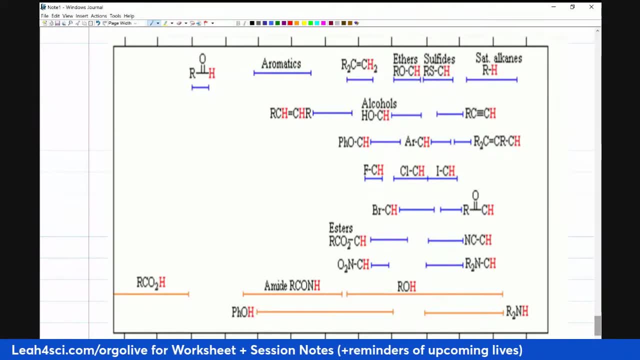 I don't know who to give credit to for this because I just Googled it, But it's basically a table or a chart like this with a lot of different functional groups looking at the chemical shift, Looking at the specific hydrogen on that functional group. 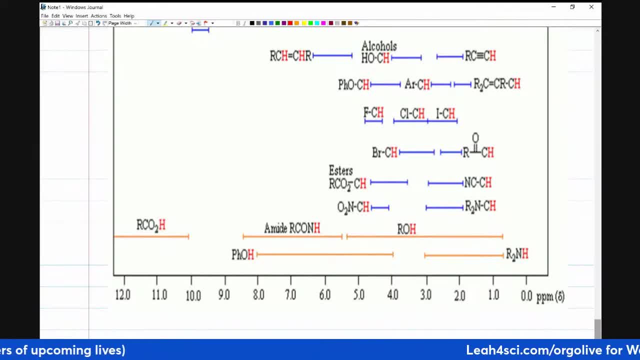 And then, where that shows up, the chemical shift for that graph. Have you taken the time to memorize this? Your professors will require you to memorize it. My problem with that, though, is: this is a lot. There's a lot going on here. 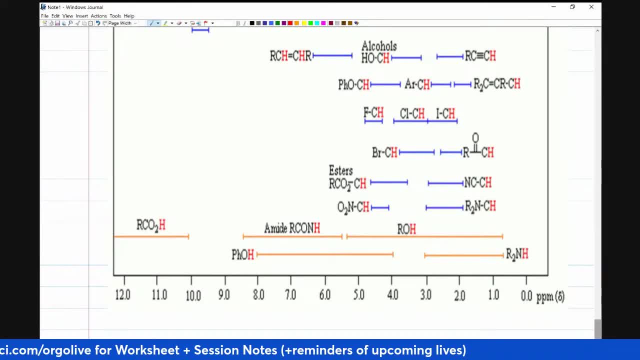 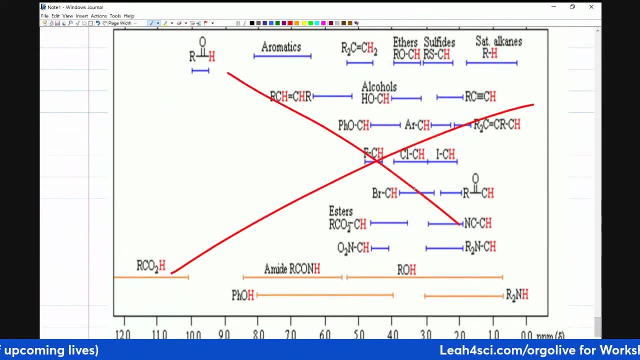 That if you try to memorize and you're just isolating- here's a number, here's a value, here's a number- you're going to be overwhelmed. So my challenge to you is to take this out of just the memorization. 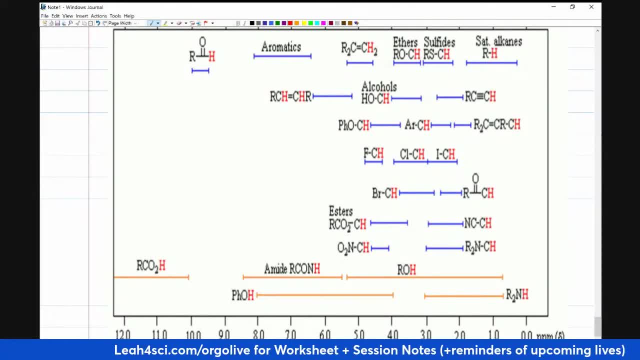 realm, And I want you to look at this more from a perspective of logic. What exactly is going on here? What are we looking at And what are the numbers actually telling us? It's not just about the fact that the hydrogen on an alcohol goes from this value. What does that actually mean? 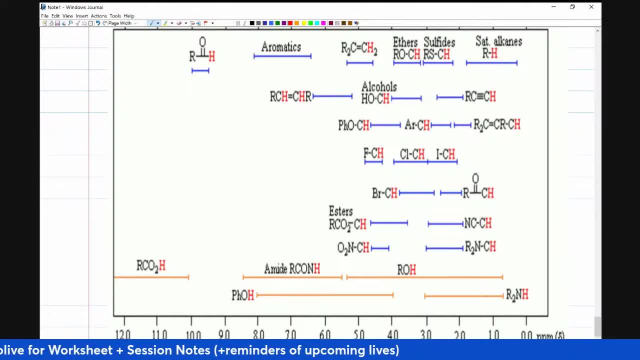 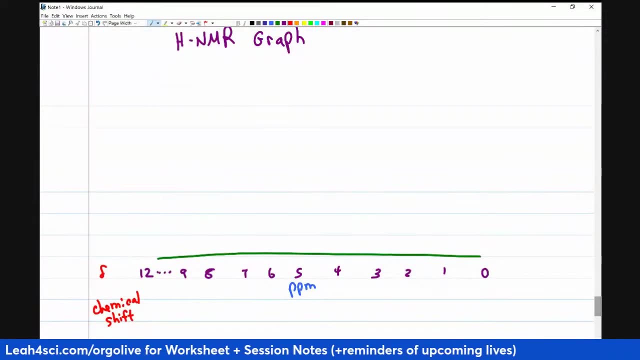 What this tells us is the chemical environment around that hydrogen. and again, not going too much into the science behind it, What I want you to understand is that if there's a hydrogen, all by itself mining its own business- for example a CH4, instead of upfield downfield. deshielded and shielded. I like to call this graph hydrogen- And I want you to understand that if there's a hydrogen all by itself mining its own business- for example, a CH4, instead of upfield, downfield, downfield, downfield. 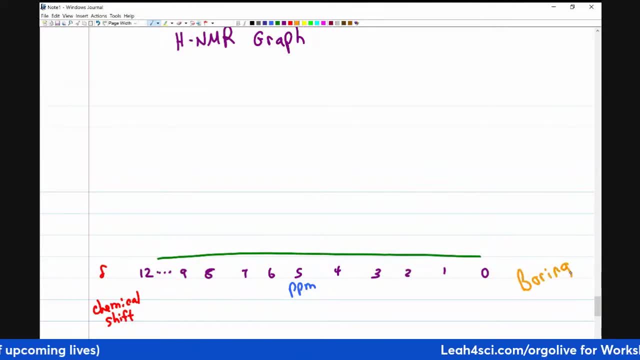 the right side of the graph boring And the left side of the graph exciting. If I have something like a CH4, just hydrogen sitting on carbon, that's pretty boring, So I would expect that to show up somewhere all the way to the right. So this would just be C to Hs. 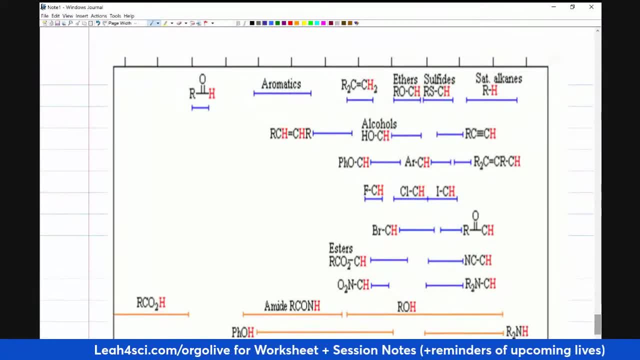 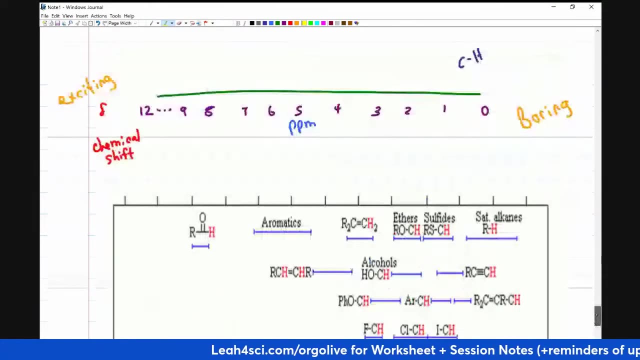 And yes, if you look at this, they're all different types. I personally can come up with a graph with a molecule off a graph faster by doing it the way I'm about to show you, rather than wasting my time with something like this, And the reason is because I understand the logic around it rather. 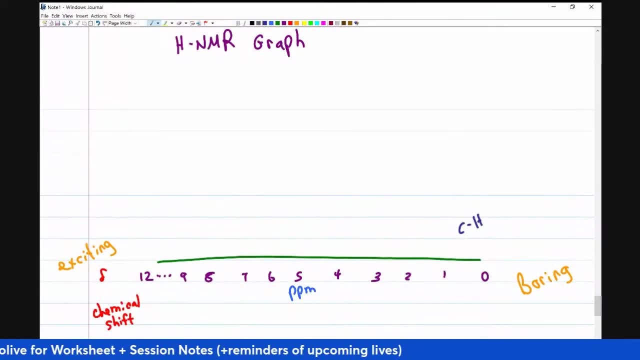 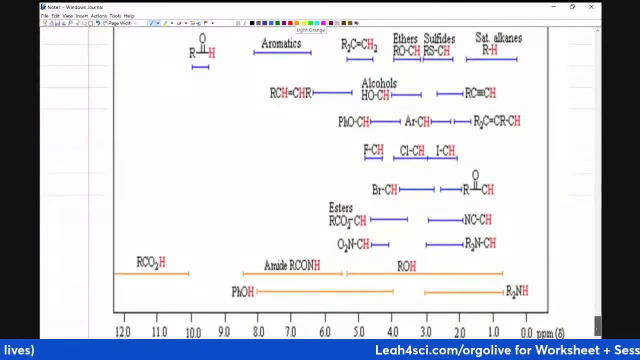 than just having memorized an exact value. So I have boring all the way over to the right, Then, and I want to show it to you on here so you can see why it ranges so much. You have your iodine, chlorine, fluorine. 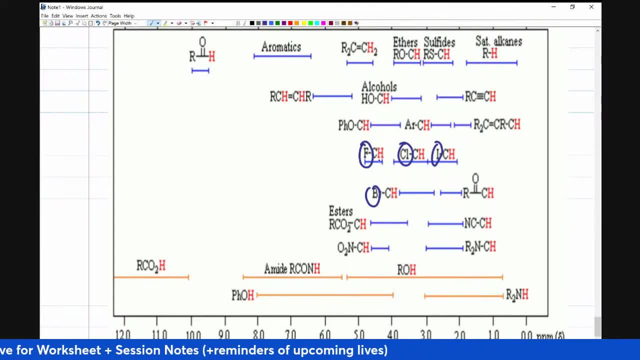 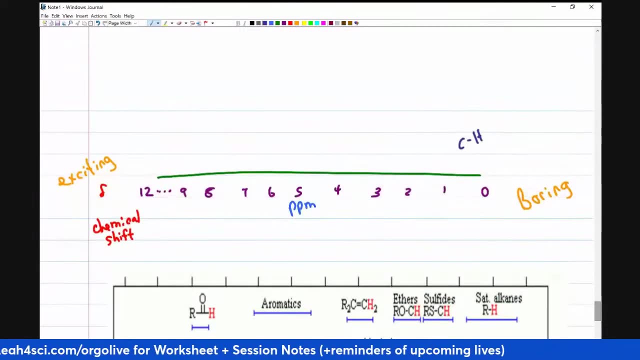 and bromine. These are your halogens, And what we're looking at is the hydrogen that is attached to the same carbon holding. a halogen Seems to range. that line is totally crooked and drunk somewhere between two and a half to four and a half, So we'll just call it the two to five range. 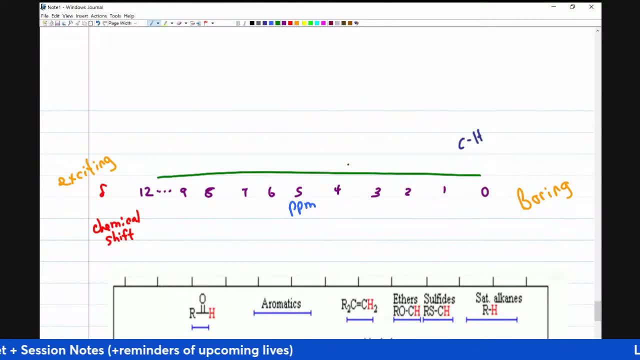 give or take, And I will just think of this range here as halogens. Which specific halogen? hopefully they give me a formula or something else to come up with it, because it's very hard to pinpoint. It's not just about that hydrogen, It's whatever is nearby, and nearby that. 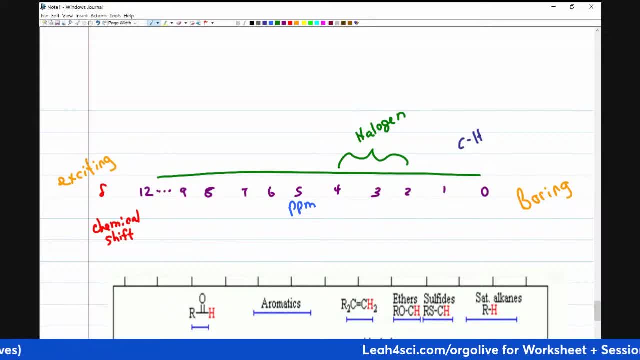 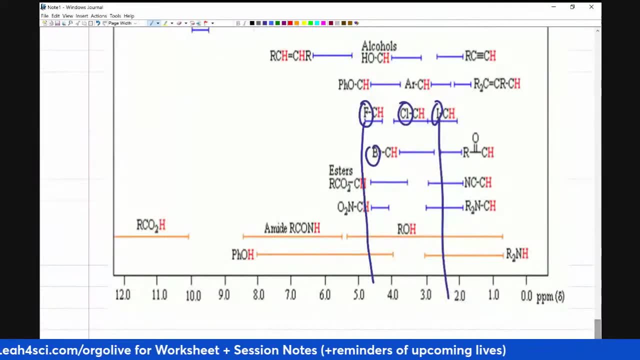 nearby that are all going to mess with it a little bit more. The next one that I recommend recognizing are alcohols and amines, And this is why memorizing the numbers is really painful. Notice the alcohol spans from about one to about five. Notice the amine spans from: 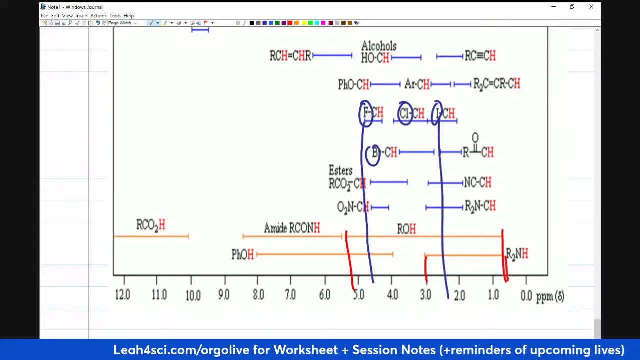 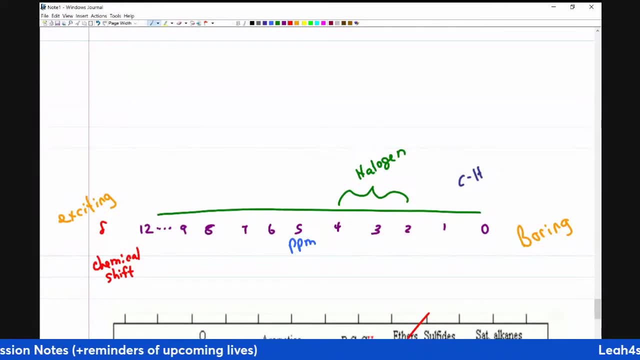 I don't even know where you read the end of this thing. about one to about three. Alcohols and amines are a bit more exciting than halogens. right It's, it's a more. the atom is less electronegative, but it's small. It's quite reactive. We see it in a lot of. 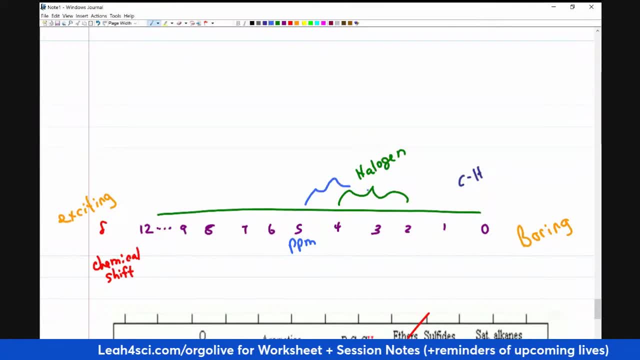 molecules. So I consider that a little more exciting, And so I tend to think of this general range of alcohols and amines as a bit more exciting, And so I tend to think of this general range of alcohols and amines as a bit more exciting, And so I tend to think of this general 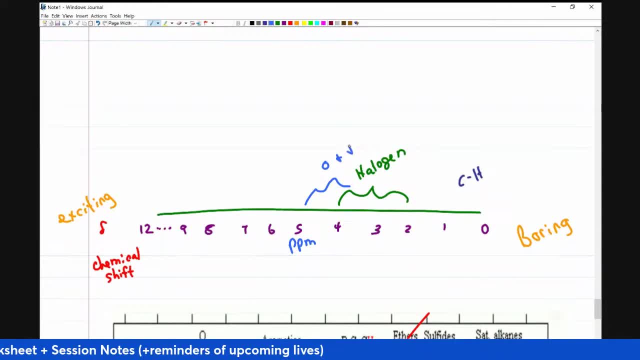 as the O and N, the alcohol and the amine. If we jump over to seven, that's where it gets really exciting. This is the general range for aromatics and pi bonds in general, but an alkene will be shifted a little bit more to the right because the benzene ring is more exciting and 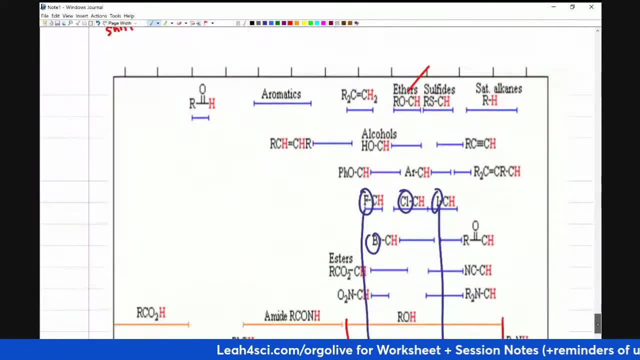 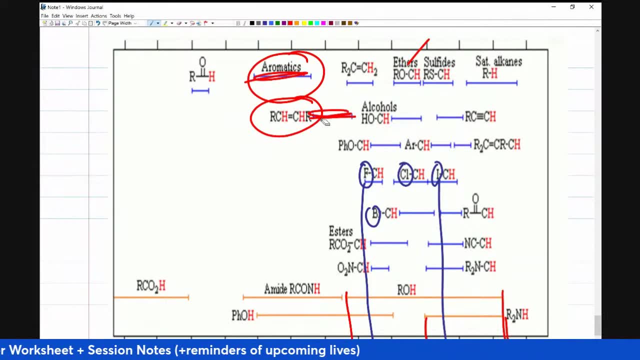 the pi bond is slightly less exciting than a full benzene ring. So let's go back to here. Notice: we have the alkene, we have the aromatic, the alkenes a bit more to the right aromatics, a bit more to the left. General direction, though about five for the pi bond. I drew that here. 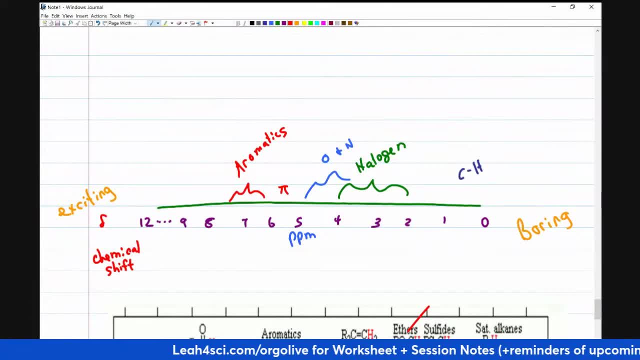 about five for the pi bond, about seven for the aromatics. And then the only other one that I highly highly recommend knowing is your carbonyl, specifically your carbonyl for an aldehyde and your carbonyl for a carboxylic acid, because these are the hydrogens. 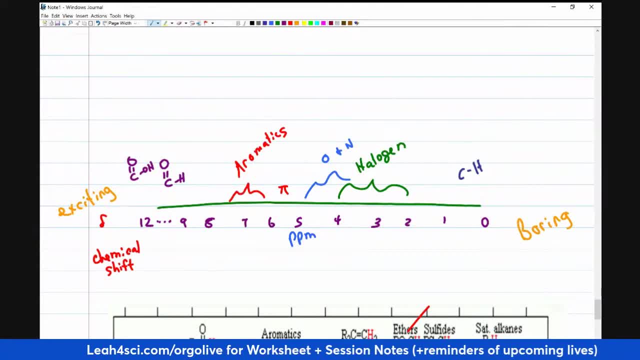 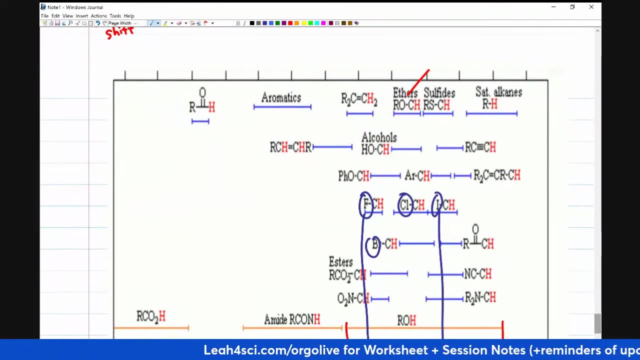 very close to that carbonyl, So not a ketone, because that will depend on whatever else is next to it. If all you're looking at is the general environment- boring and exciting- does this feel easier to memorize than this right here? And if it does and you haven't yet subscribed to my 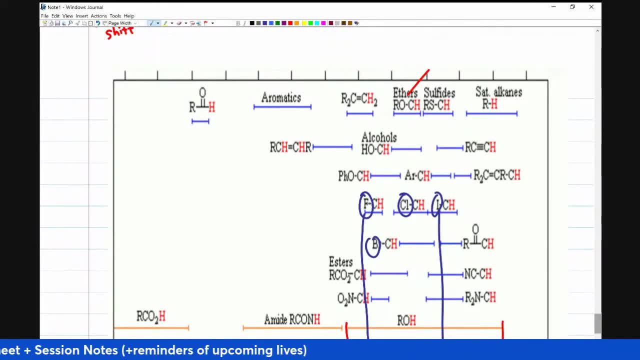 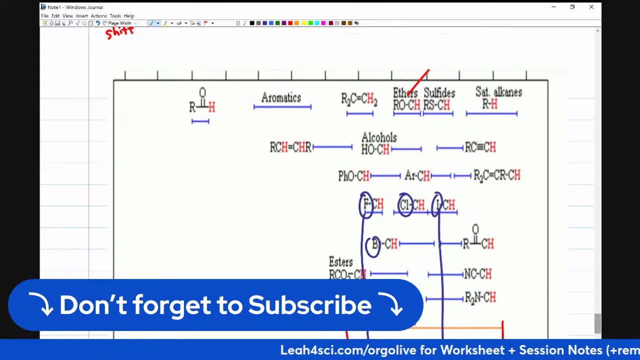 channel. what are you waiting for? Hold on, I have a button for that. It's my first time using these buttons, so I'm just playing around with them, All right. so let's see if we can take this information, the simpler approach to all of this, and make some kind of sense around it. 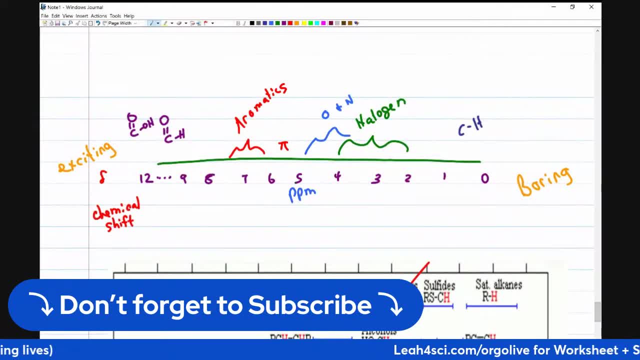 Actually, before I show you another example, another peak that you may see is around zero. You'll see a line here. Sometimes you'll see TMS written on it. This is simply the zeroizer, the thing that helps set the baseline for let's find the TMS. 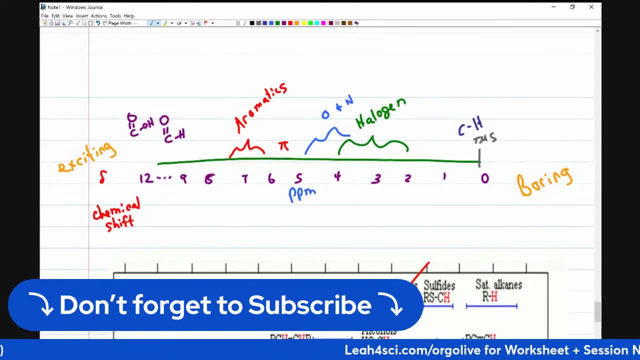 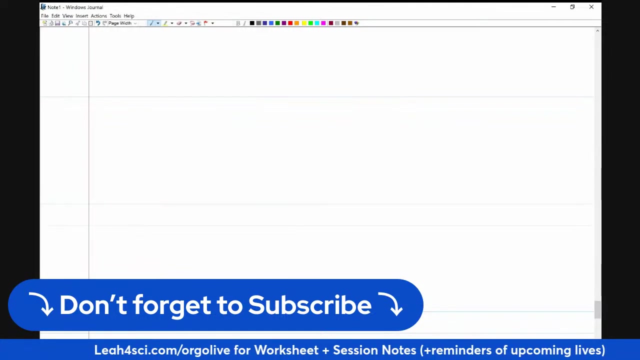 and solution. We set this to zero and, based on this, the machine will create the scale to show you everything else. Are you ready to put it all together? If you are, let me know in the comments. We'll start with a couple of simple examples and then I'll tell you where I have more. 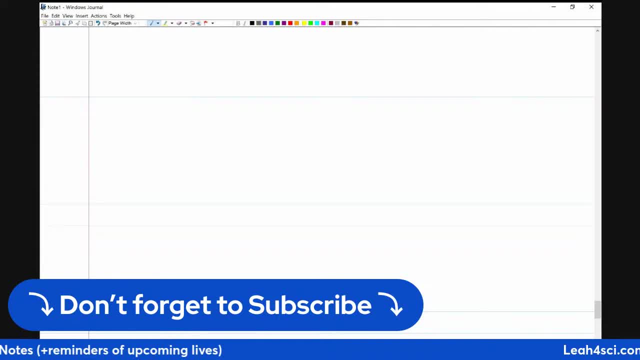 where we do more. So let's go ahead and start with the first one. So for the first one we're given the molecular formula C2H5O and then we're given a graph that looks like this: The graph only goes from zero to four, and on the graph we have a total of 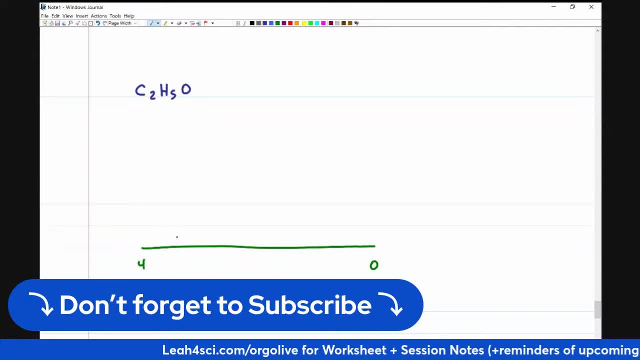 three peaks. Just under four. we have a quartet- I did not draw that right- Just under three. oh, I should give you more numbers, shouldn't I? Four, three, two, one. So I'm exaggerating these a bit because I want you to clearly see what I have drawn on the screen. 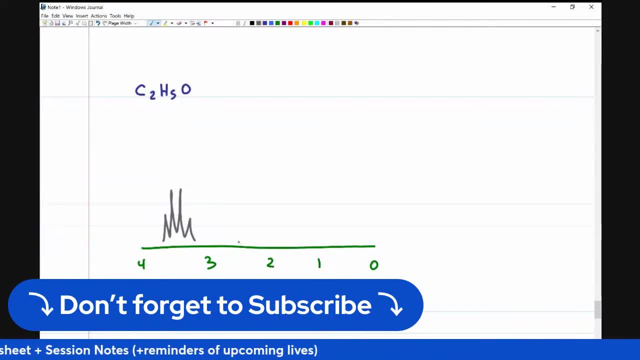 Sometimes you need a magnifying glass for these things. Under three, we have a singlet, And a little greater than one, we have a triplet. Okay, That is all the numbers. that's provided, And what you have to do is come up with a molecule, come up with a structure for. 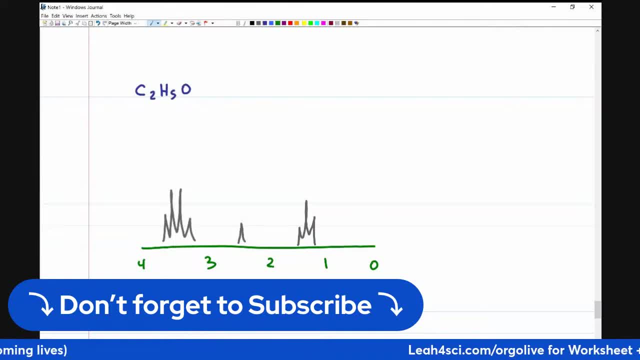 what we have written on this graph. What is your first step to figuring out what we have here? Before you even look at the graph, I want you to have a general idea of the direction that you're going, Because if you need a ring or you need a pi bond, you want to know that up front And the 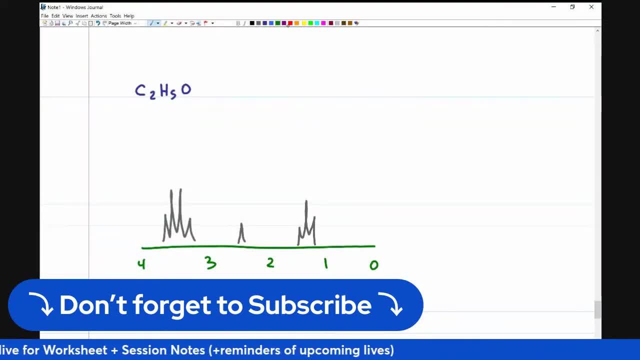 way to know that is by figuring out the index of hydrogen deficiency. So step one is find your index of hydrogen deficiency, And I have a video that teaches you how to do this, linked in the description, or will be linked in the description if you need to review that later, But we're going. 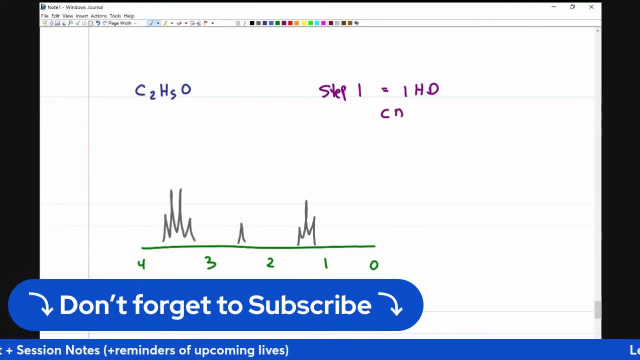 to use the equation of C N, H2N plus 2 to figure out how many pi bonds or rings we potentially have in the molecule. C N is 2.. Now, this is a different N than neighbors. This is just the number of carbons that we have. 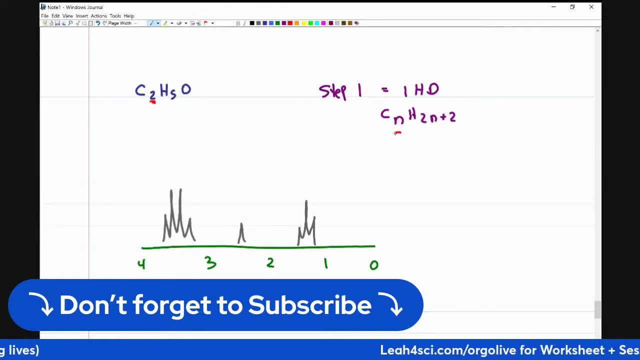 to figure out the ratio of hydrogens. And so if N is equal to 2, then 2N plus 2,. 2 times 2 is 4 plus 2 is 6.. We should have a total of oh. 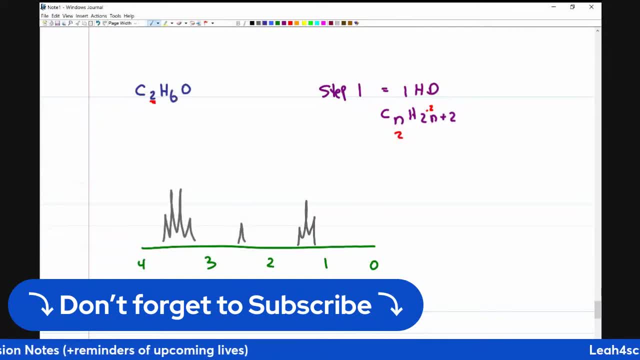 I missed sorry. that should be a 6.. We should have a total of 6.. 2N plus 2 is equal to 6.. We have 6.. So 6 minus 6 equals 0.. 0 pi bonds, 0 rings in the molecule. That makes it easier. I have a. 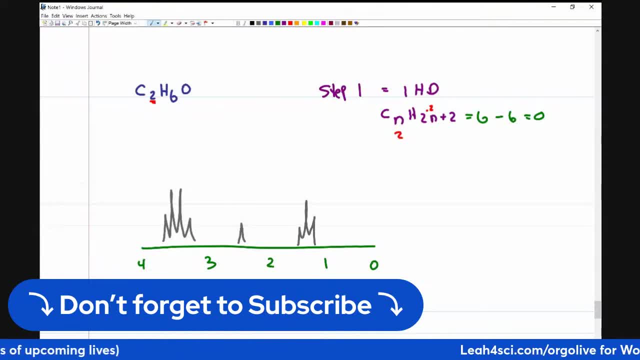 fully saturated molecule. So let's figure out the next step. What I'd like to do here is see if the molecule itself can give me any clues. Meaning: is there something obvious, Instead of just trying to draw structures and guess? I might do this one. You could probably guess easily, because it's only 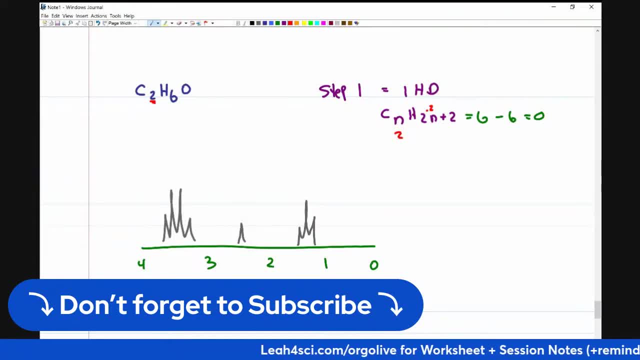 two carbons. You could just draw different isomers, But what I like to do is have a general idea of. is there something on the molecule that is on the graph that is giving me a clue? For example, I have a singlet. 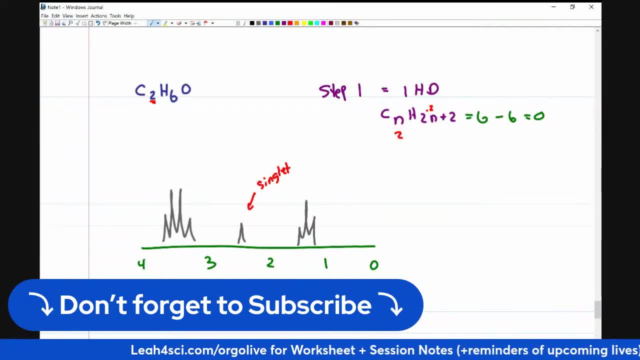 The singlet tells me there's no splitting. I want to keep that in mind. The next thing I have is a quartet, And let's make each of these different colors so that we can then match it up to the molecule. How many neighbors does this quartet have? 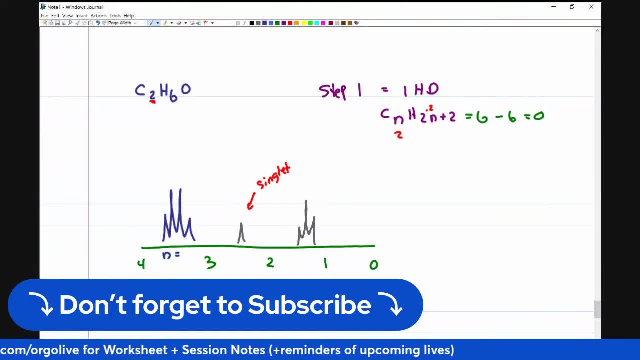 N equals what Well we count the peaks, We have a total of 1,, 2,, 3,, 4.. N plus 1 gives me the number of peaks, And so 4 tips minus 1 equals 3.. 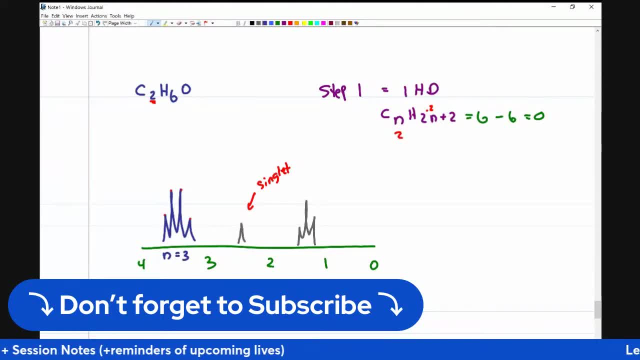 N equals 3.. There is something on this molecule that has 3 hydrogens. It's not the blue one. Whatever carbon I designate in blue doesn't have 3 hydrogens- The carbon attached to it. and this I want to make sure you're very clear. 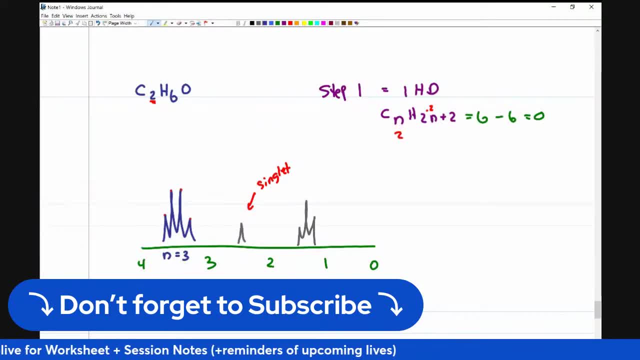 the carbon attached to whatever is here. that is the one that has 3 hydrogens. Let's do the same thing over here. We'll make this one purple. And what do we see over here? 1,, 2,, 3.. 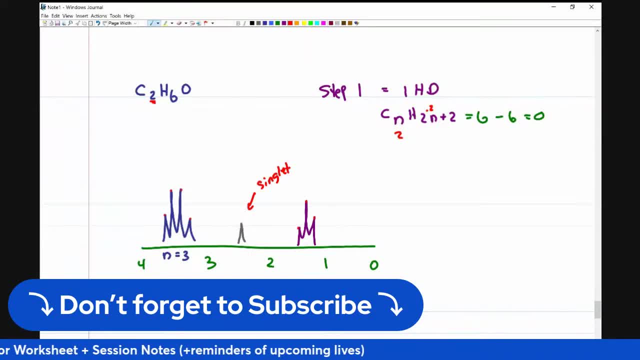 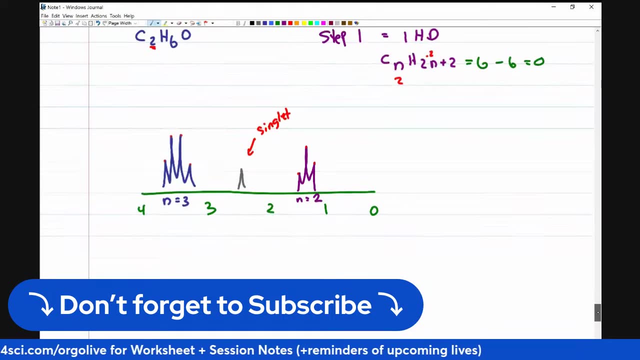 3 tips total right in the peaks. N plus 1 equals 3.. N is equal to 2.. That means, whatever I draw in, purple has 2 hydrogens. Now this is where the puzzle starts to come together. I'll show you a trick for this after, but here's what we're looking at. 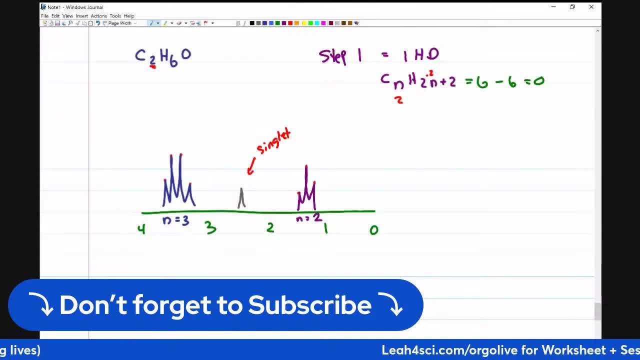 Somewhere on the molecule. I have a carbon that has 3 hydrogens. That means there is a CH3 on the molecule. It's not this. There's a CH3 somewhere else on the molecule. So let's put a CH3 right here. 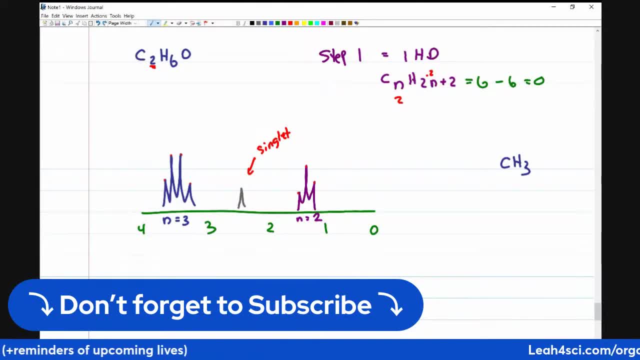 Somewhere else on the molecule, I have a carbon with 2 hydrogens, That is, a CH2.. What I like to do now is do some quick math. If I have C2H6O, C2H6O minus these two, 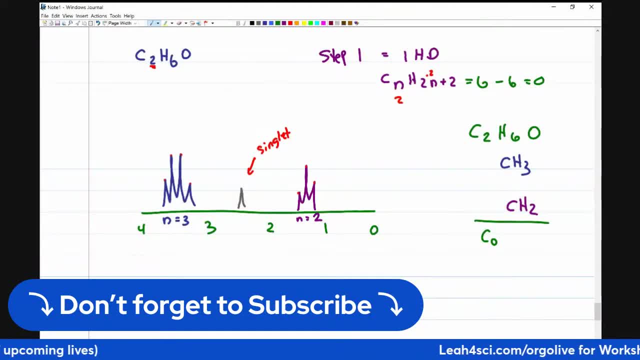 well then, I should have C0,. all my carbons are accounted for: H1 and O1. That means an OH is the only group unaccounted for, And that is my other piece. I treat this as a puzzle. And so what do we have? 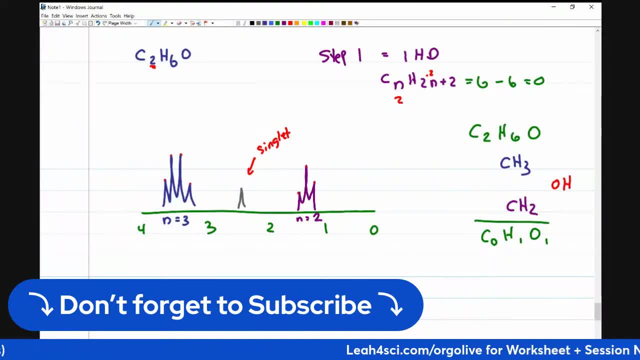 I have a CH3.. The only possible bond on a CH3 is to carbon. A CH2 can have a total of 2 bonds, So I have a CH3.. The only possible bond on a CH3 is to carbon, So I'm going to bind it to this CH3. 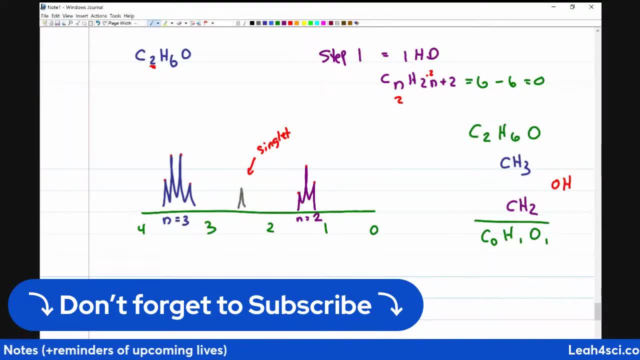 And then where did I put that? And then, attached to that, we'll put the OH. But wait, I did that backwards. The CH3, notice that the CH3 is actually this peak Because it has 2 neighbors. The CH2 is that peak. 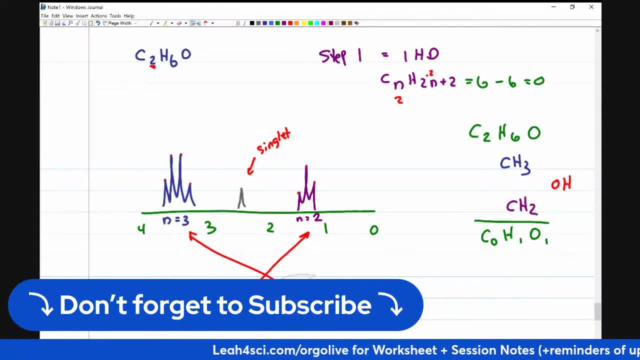 I got my colors backwards. This should be the purple group, This should be the blue group. Do you see why I switched them? Do you see why the colors are backwards? Whatever it is that had 3 neighbors is blue. What has 3 neighbors? 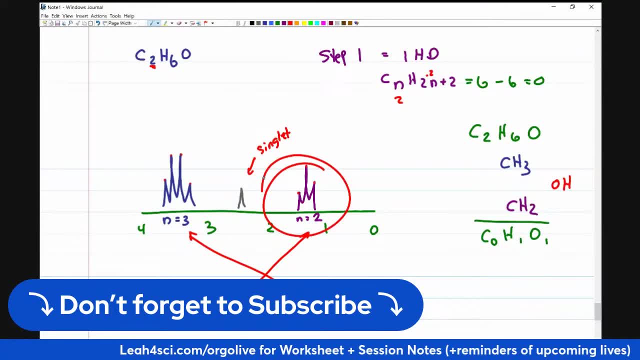 The CH2.. Whatever it is that had 2 neighbors is purple. The CH3 has 2 neighbors, It is purple, And then the hydrogen is going to show up as a singlet All by itself, Even though the hydrogen on alcohol 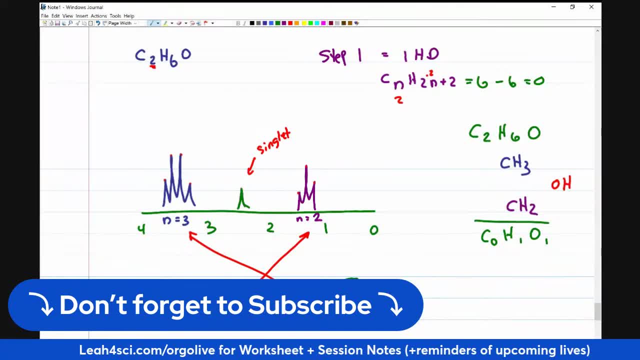 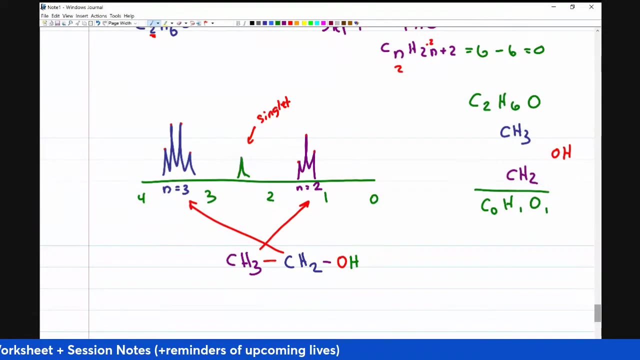 no matter what is next to, it is going to be a singlet all by itself. And that is my final answer: Ethanol. Let me know if that's better, All right, So let me show you another trick that I want you to recognize. 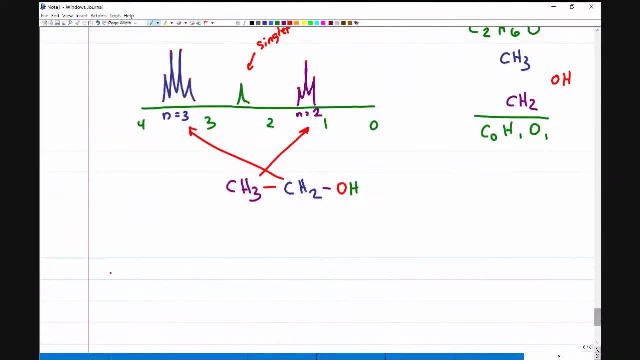 I want you to look for the pattern that I show you here, And that is anytime. you see, just standing out, if you have a quartet and a triplet, where the quartet represents 2 hydrogens and the triplet represents 3 hydrogens, 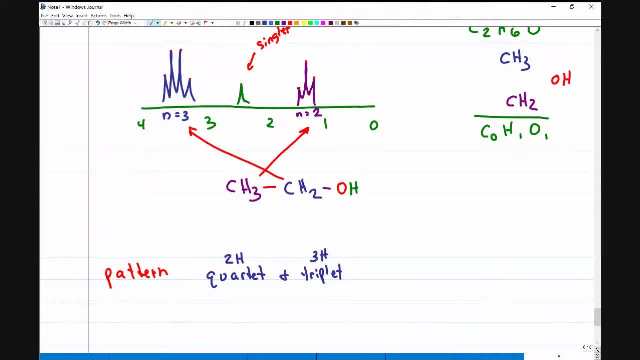 Here I didn't show you, but on some of the molecules you will be told, this represents X number of hydrogens. This, right here, means that you have an ethyl group, A quartet, a triplet. notice: they neighbor each other, They split each other. 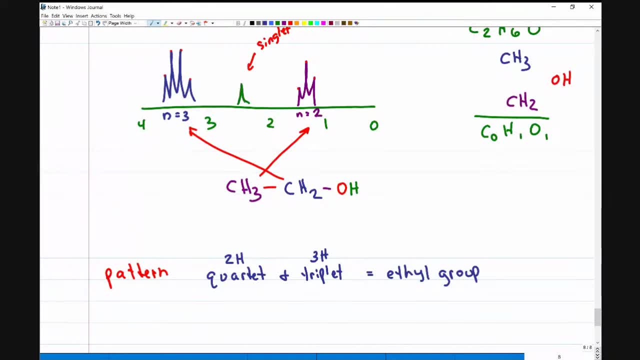 So if you see a quartet and a triplet, ask yourself: do I potentially have an ethyl group on this molecule? And if yes, look for it and see if it matches up. If you have any questions on this, go ahead and type it in. 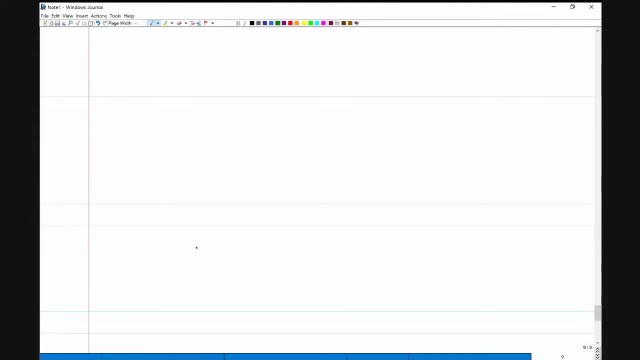 while I draw out the next one. The next one is also a shorter graph. This one goes from 0, 1, 2, and 3.. And on this graph we have between 2 and 3, there is a quartet. 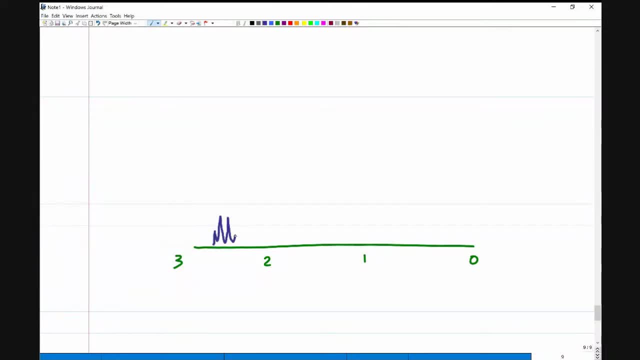 Why is it doing that? Just after 2,, we have a tall singlet Trying to make it skinny- Eh, close enough. And then, just after 1,, we have a triplet. The molecular formula that we're looking at is C4H8O. 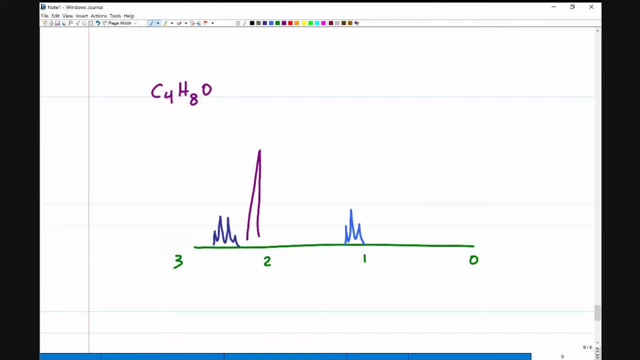 What is the first step in solving a molecule like this? The first thing we have to do before we look at anything else is find the index of hydrogen deficiency. If we're using the equation CnH2n plus 2 and n is equal to 4,. 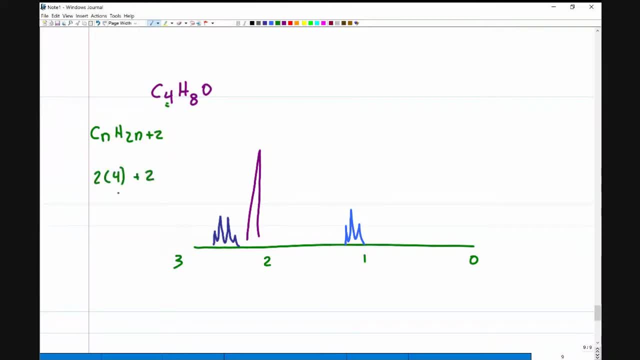 then 2 times n plus 2, 2 times 4 is 8 plus 2 equals 10.. We subtract what we have minus 8 gives me 2.. When you're looking at the index of hydrogen deficiency, every 2 is 2 hydrogens missing. 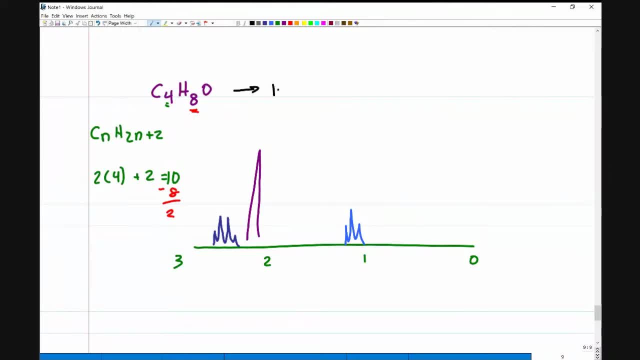 for a pi bond or a ring. And that tells me the index of hydrogen deficiency is equal to 1.. And that means 1 pi or 1 ring. This is where it can get a little bit tricky. Am I missing a peak on this? 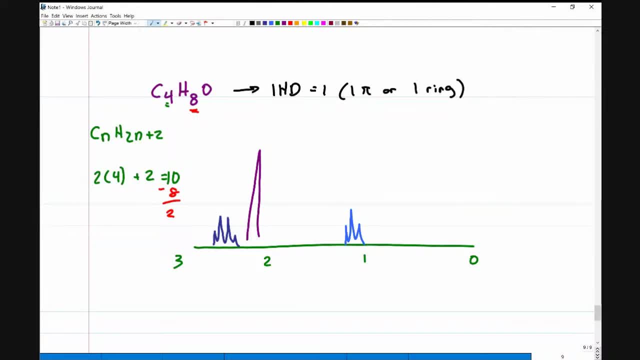 No, I'm not Okay. So here is another approach I like to take. as the molecule gets bigger, I want you to try to assign a carbon to each of these, So we can say that we have whoops, that we have a blue carbon. 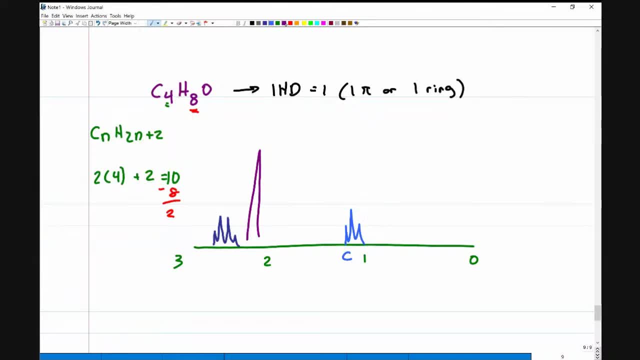 that is responsible for this peak. We have a purple carbon responsible for this peak and a dark blue carbon responsible for this peak. That gives me 3 carbons. The fourth one is unaccounted for. This helps me figure out that what I have. 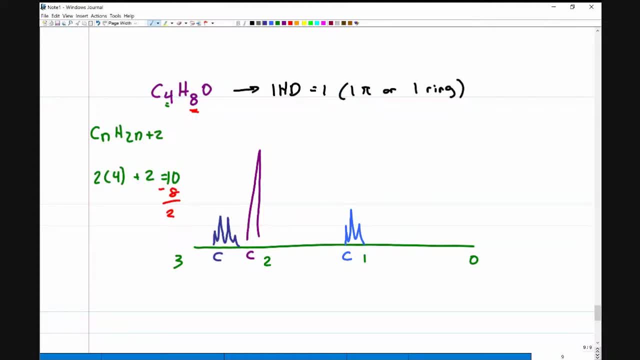 is probably a pi bond. So let me talk you through the logic here. If a carbon does not show up on the HNMR graph, it means the carbon has no hydrogen. If carbon is not on the graph and there's no symmetry in the molecule, 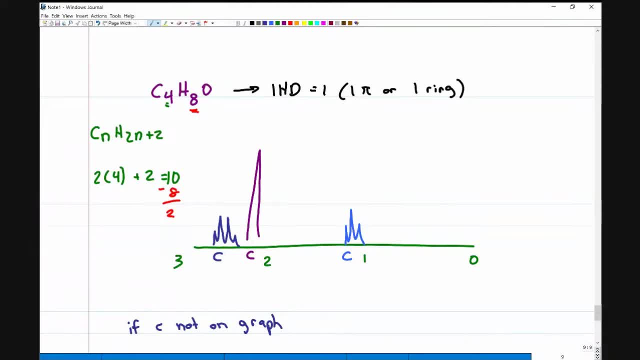 in this case there is no symmetry. I'm assuming no symmetry based on how it's presented. So if carbon is not on the graph, it has no hydrogen. What would be an example of a carbon that doesn't have a hydrogen? A carbon with 4 carbons? 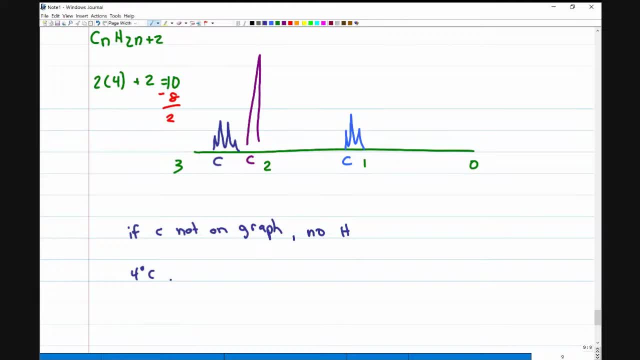 coming out of it. so a quaternary carbon, meaning carbon bound to just a bunch of other things, or a carbonyl, is another example. A carbonyl that is then bound to carbons on either side does not have a hydrogen. 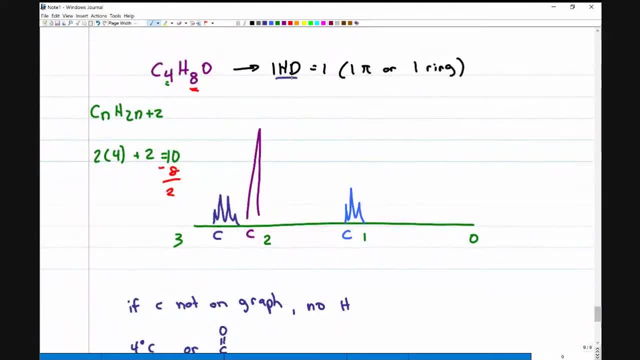 to show up on this graph. If we have an index of hydrogen deficiency- meaning we have a pi bond or a ring- I have an oxygen and I don't see any evidence of the oxygen on the ring. So when I know there's an oxygen, 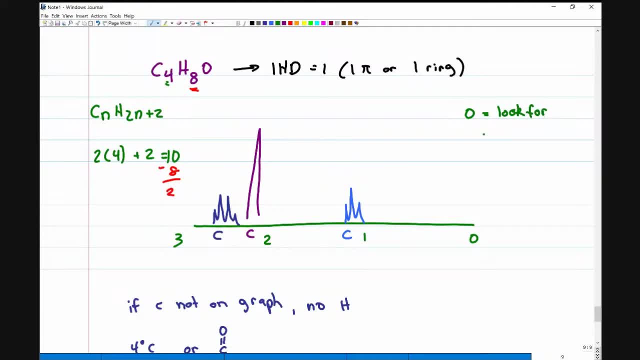 what I want you to do is look for the 9 to 12 range to see if we have a carboxylic acid, an aldehyde or the less than 5 singlet- And this is a small. typically the alcohol shows up like that. 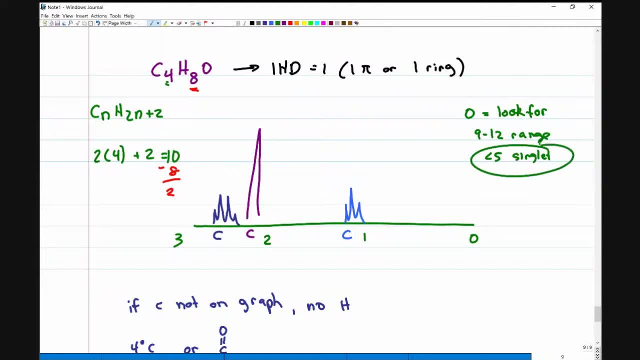 So this would be your carboxylic acid and aldehyde. This would be an alcohol, but I don't have any of that. So, in seeing that I don't have anything obvious for the oxygen and I have a pi bond and I have a carbon unaccounted for, 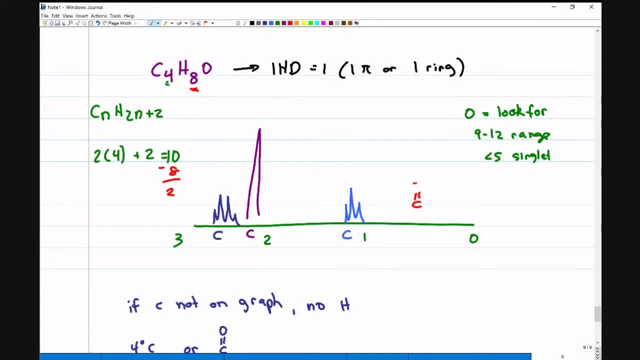 I'm going to say that my fourth puzzle piece is a carbonyl And that is everything I have on my molecule: The blue group, the purple group, the blue group, the light blue group and the red group. So let's start putting it together. 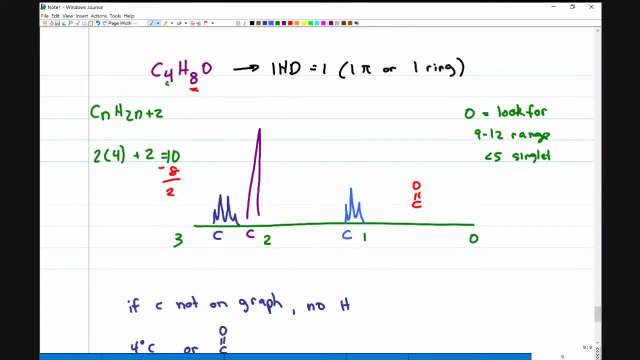 in terms of the pieces, I already have one piece. This one right here is a singlet. The singlet means that it has no neighbors. N equals zero, So that means it has to be attached to something that does not have hydrogens. 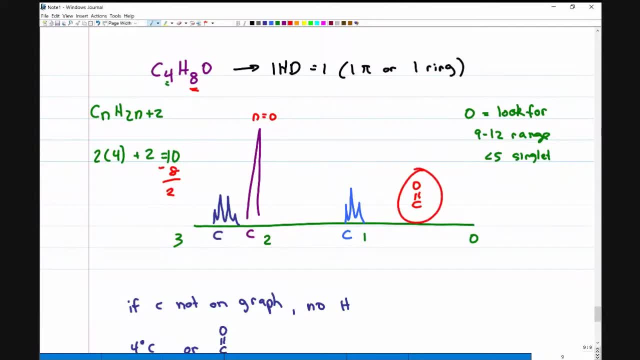 Well, what on? this molecule has no hydrogens- My carbonyl. So let's start putting the puzzle together up here. If I have a carbonyl and attached to that I have a carbon with no hydrogens next to it, or a carbon with a peak, 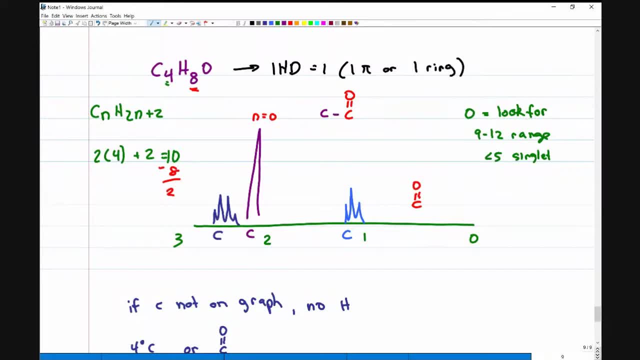 that is a singlet. How many hydrogens would this have to be? It has to be three, Because if there's nothing else attached to it, well, I have to fill up every bond. So I already have two of the four carbons. 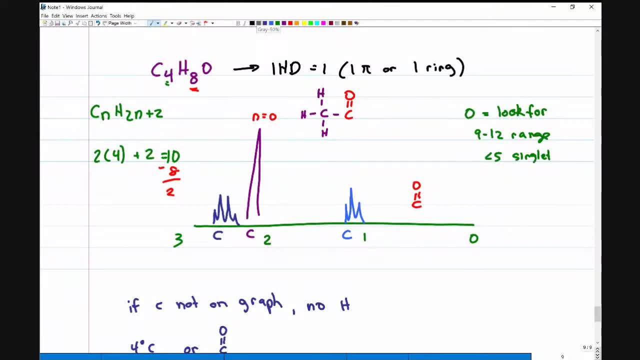 and now I'm left with. well, I have to find the other two. Look at the pattern: A quartet and a triplet. What should automatically come to mind if you see a quartet and a triplet? We're looking for an ethyl group. 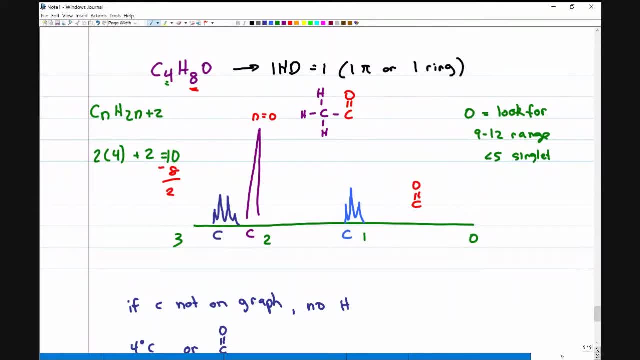 So let's see if we can justify it. If the dark blue has one, two, three, four, That means four minus one equals three, N equals three. It has three neighbors. That means whatever this blue one is probably has a CH3. 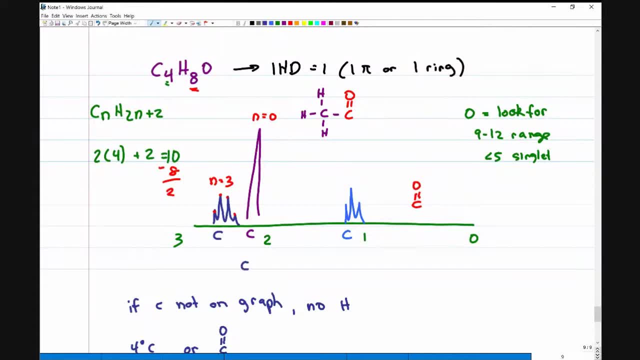 next to it. So this blue carbon can have a ghost CH3 next to it. The light blue one, two, three, Three minus one equals two, N equals two. That means it has a CH2 next to it. So this light blue carbon. 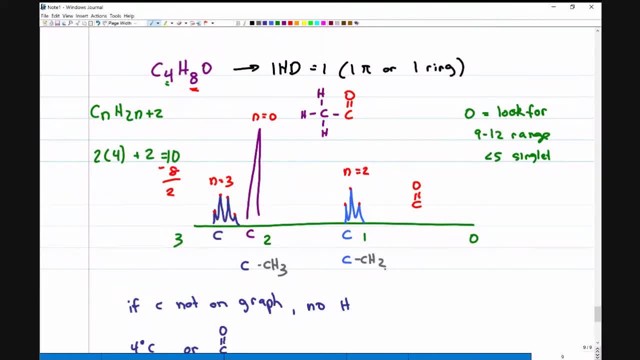 has a ghost CH2 next to it. Can we then assume that this is a CH3 and this is a CH2?? Well, yeah, it fits perfectly. So this would be the dark blue is my CH2 because, remember, it has a CH3 attached. 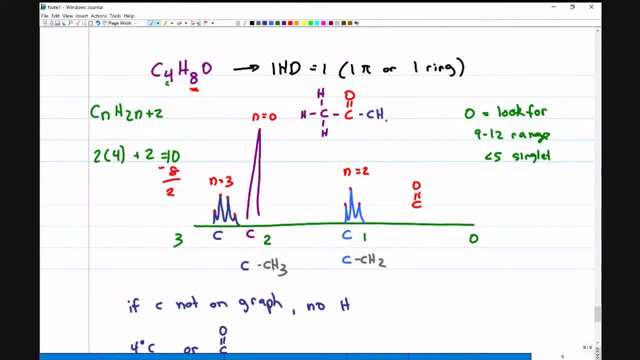 The light blue. why do I keep doing that? The light blue is a CH3 because it has a CH2 attached Again. this is: this is the CH3 because its neighbor is a CH2.. It's not the CH2 itself. 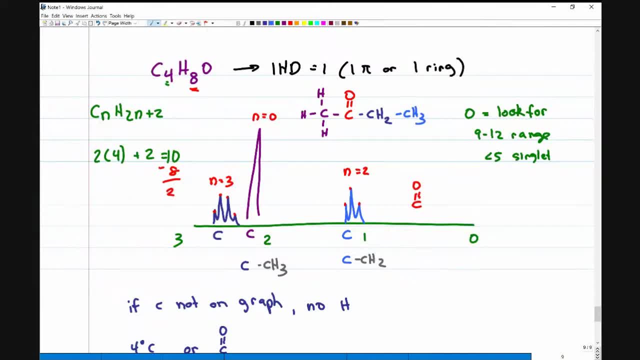 Its neighbor is the CH2.. And I want to justify it based on the concept of boring and exciting on the graph, If you look at the way the molecule is written, and oh my goodness, this is a real mess. Let's see if we can get. 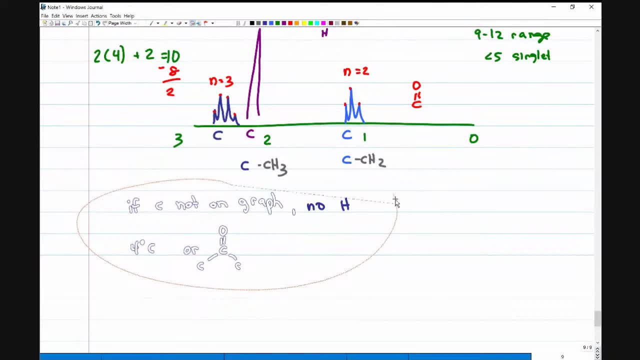 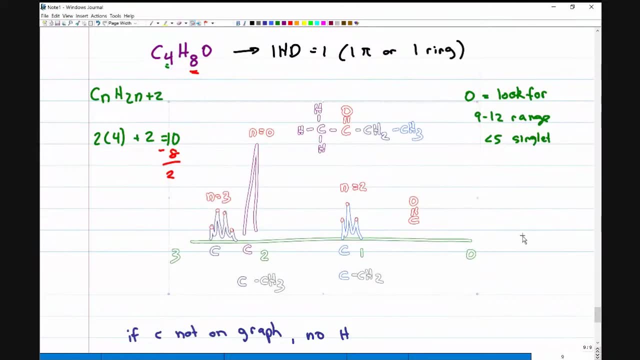 some of this just out of the way. Let's move this down. I want to isolate it a little so that we can clearly see what we're looking at. Notice that the most exciting thing on this molecule is the carbonyl. That means 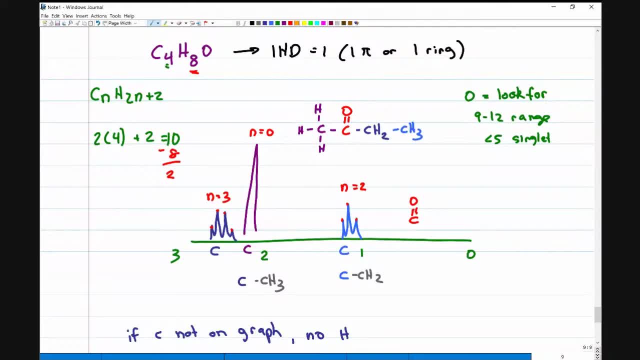 anything attached to the carbonyl would be exciting. This purple group and this blue group- dark blue- are attached to the carbonyl and notice they're both shifted to the left, where the CH2 is more exciting than the CH3. It's the furthest. 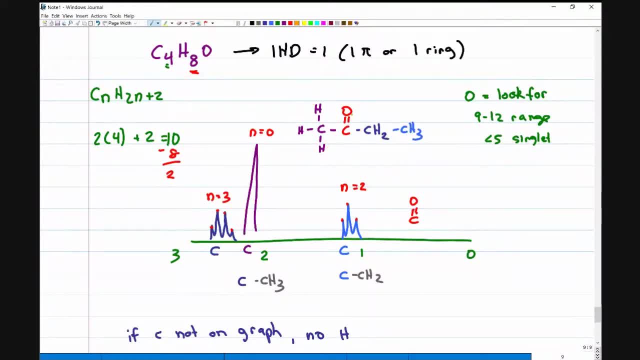 to the left, and the reason it's the most exciting is it has a carbonyl on one side and something else on the other side, where this one has a carbonyl on one side and nothing else. Slightly less exciting Now this CH3. 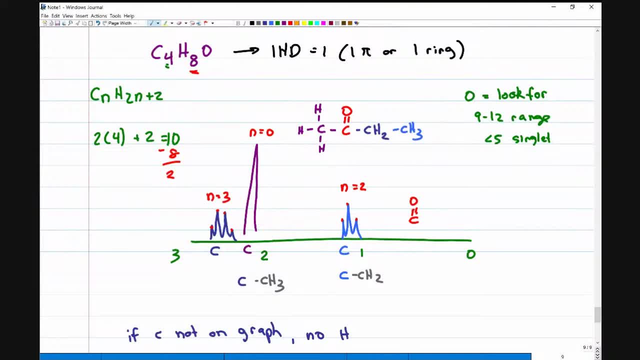 is sitting on a CH2.. Not much going on, but its neighbor is to the neighbor of something exciting and so it's not completely in the boring dead zone But shifted just a little bit out of the boring zone. still kind of boring Question. 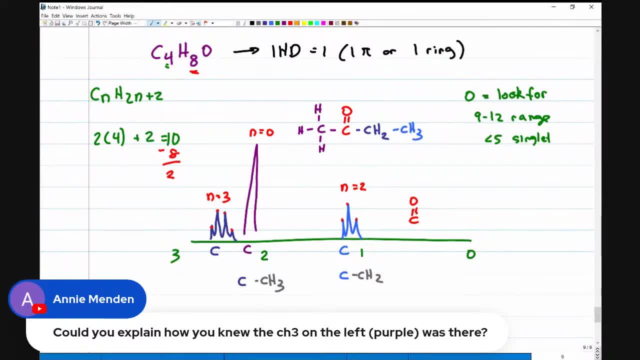 Can you please explain how you knew the CH3 on the left was there? In looking at the graph, the first thing I did after finding the index of hydrogen deficiency was assign a carbon to each peak, And so I knew that the purple represented a carbon. 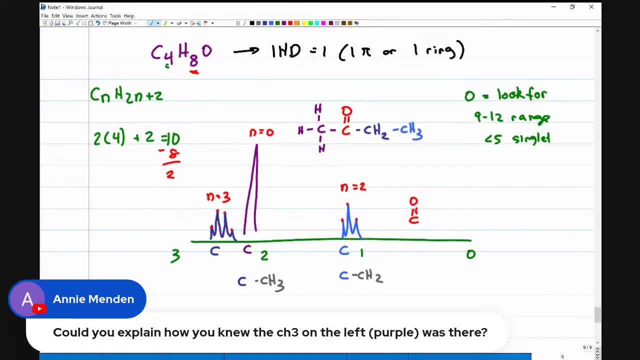 and because the purple has a singlet, it has no neighbors. Given that we already predicted a carbonyl on this molecule, the only way to have no neighbors is to have the purple carbon attached to the carbonyl, which doesn't have hydrogens. 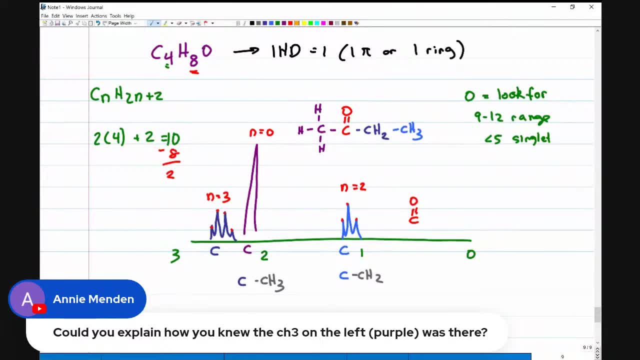 and then nothing on the other side, because if I put something on the other side, it would have nothing on the other side. So I knew that the purple represented a carbon and because the purple has a singlet, which is if I put something on the other side. 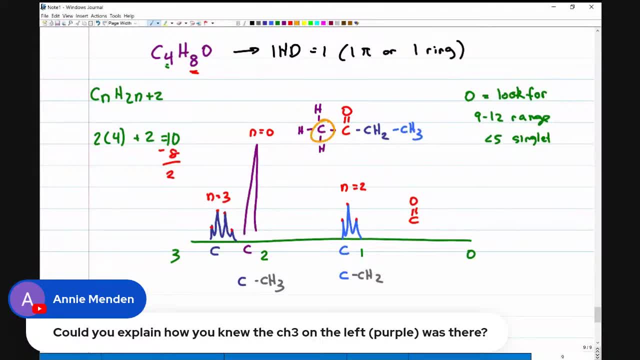 it would have neighbors Once I knew that the purple carbon was sitting at the end of the molecule, next to this. that completely cuts it off. it had to be a CH3, because the only way to have a complete octet on a terminal carbon is to give it. 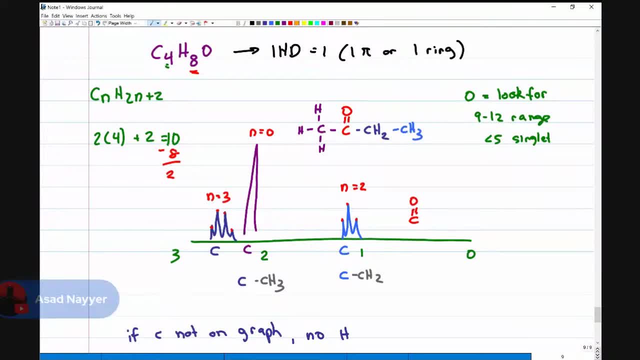 three hydrogens. That was a very good question. I hope that's clear. How did you know it was a carbonyl? again, This was a very educated guess and here are the clues that I saw. Here are the clues I want you to look for. 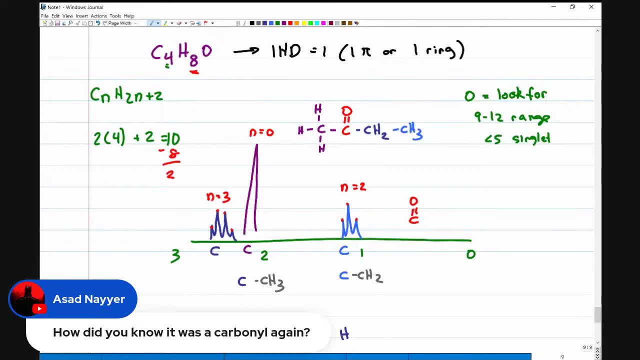 I have a small molecule with an index of hydrogen deficiency equals one, One pi bond and one ring. What I didn't tell you before is that I ruled out pi bonds like a carbon to carbon double bond, because there's nothing in the five to seven range. 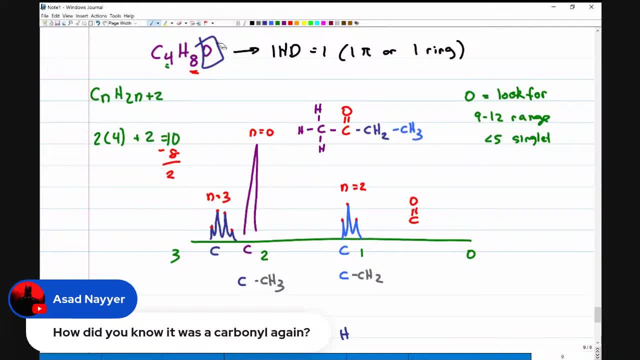 I know that I have an oxygen and the oxygen doesn't have an obvious functional group. I don't have anything in the nine to twelve range telling me carboxylic acid or aldehyde. I don't have a broad, small singlet telling me. 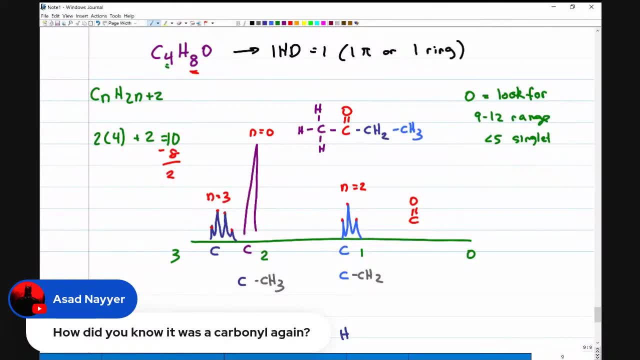 a potential alcohol. Now the oxygen could have been an ether as well. That is another option. But if I had an ether then A, I would have to have a pi bond there as well, because my index of hydrogen deficiency would still have to be. 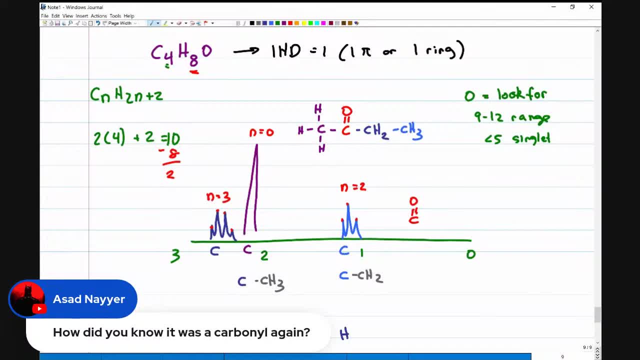 on the molecule. So I'd have to have a pi bond and I would have to have all four carbons having hydrogens. So the only way to have an index of hydrogen deficiency and completely hide a carbon from the HNMR graph is if it has no hydrogen on it. 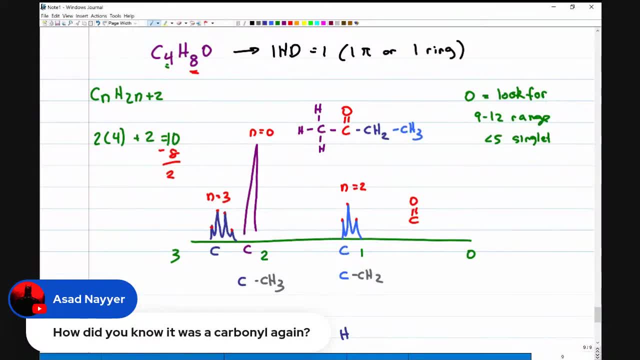 So, taking all those things together, I determined that I likely have a carbonyl. So I know I was talking a lot. Let's see if we can summarize it. Index of hydrogen deficiency. No obvious pi bond. You're missing a carbon on the graph. 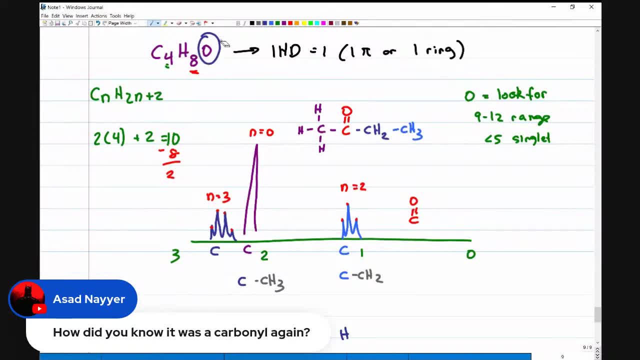 You have an oxygen without an obvious functional group for it. Those are the clues that I look for. Are you comfortable with everything that I showed you today? Are you comfortable with how to approach this And if yes, do you want even more practice? 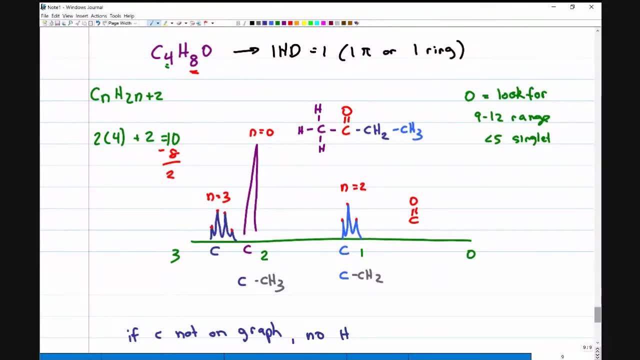 So I'm seeing yes and yes. What I'm going to do is the additional problems that I wrote out First. I'm going to provide the worksheet, So if you sign up, the link is on the screen. Let me put it in bigger.